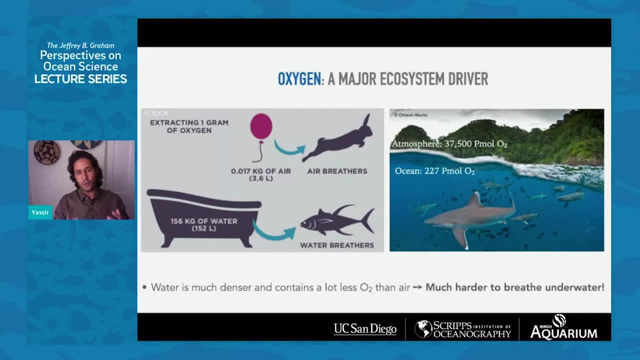 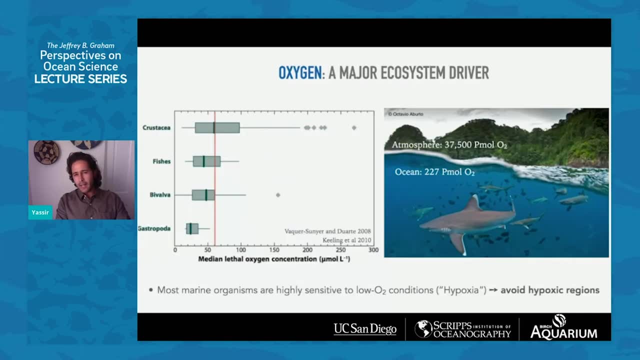 you can get the same amount of oxygen, So it's really hard to breathe. It's not as abundant And there are values of oxygen that are detrimental to fish health, and they exist throughout the ocean's interior, in certain parts of the Pacific, for example, And these are called hypoxic. 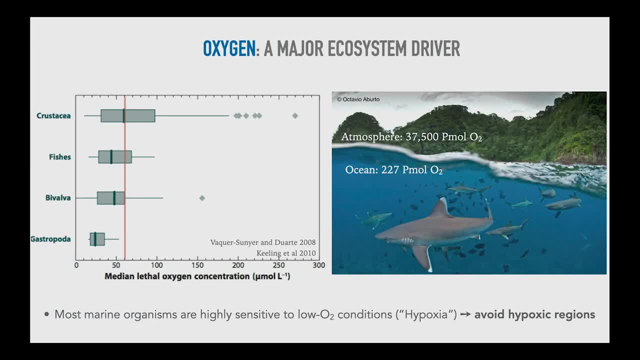 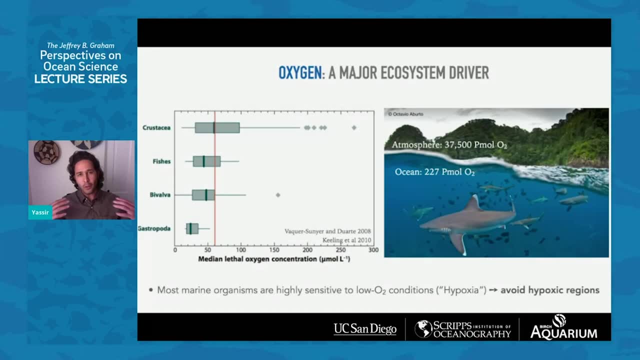 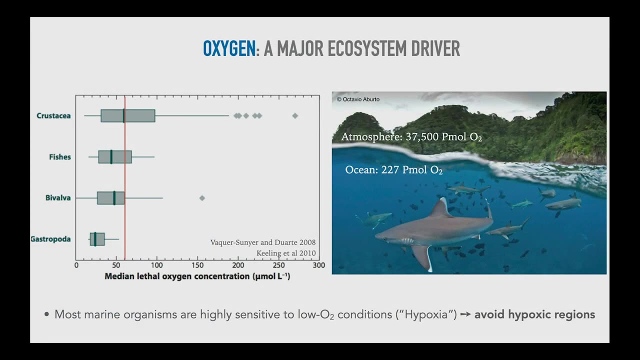 conditions. These are values of oxygen where, when they reach about 60 micromole per liter or less, marine organisms start to feel severe physiological changes. It's like humans without air And that's going to depend on whether you're a crustacean, like a crab, or a fish, or a bivalve or a gastropod, And you can see here in the plot to. 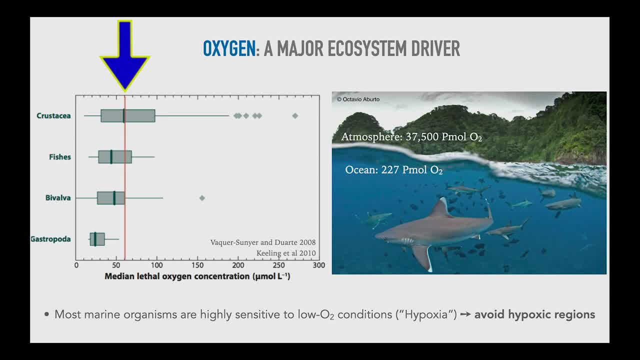 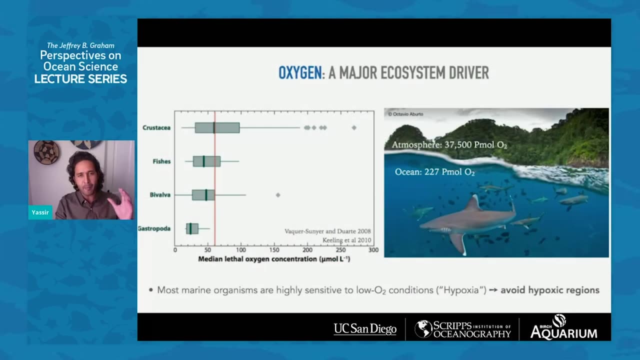 the left to my left, you see that right around 60 micromole per liter is that hypoxic depth below which many organisms begin to feel this hypoxic conditions. So, throughout the oceans, marine life is going to avoid this hypoxic condition and that's going to set up their 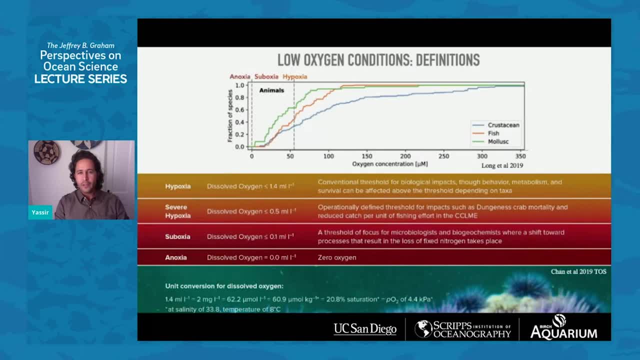 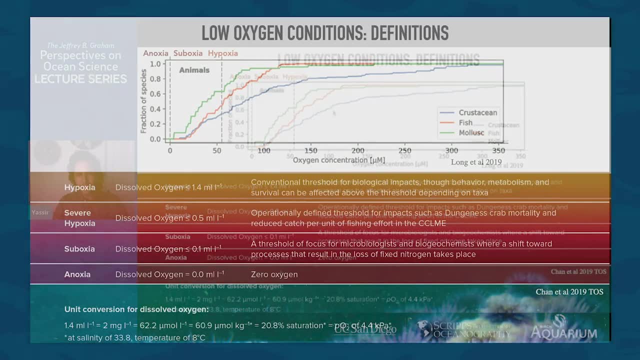 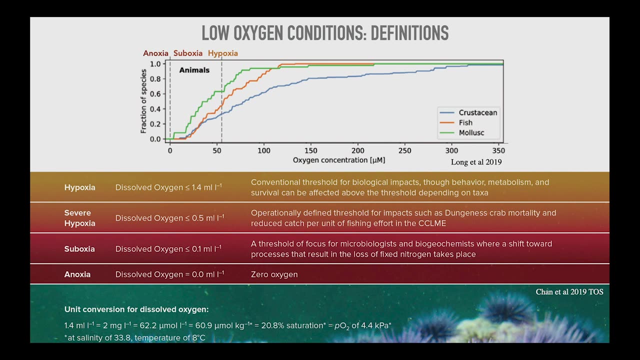 marine ecosystem habitats. So how much of marine organisms can survive below or above? You could see up here this figure shows in green the fraction of species of mollusks, or in orange the fraction of species of fish, or in blue here the fraction of species of crustaceans that can live below. 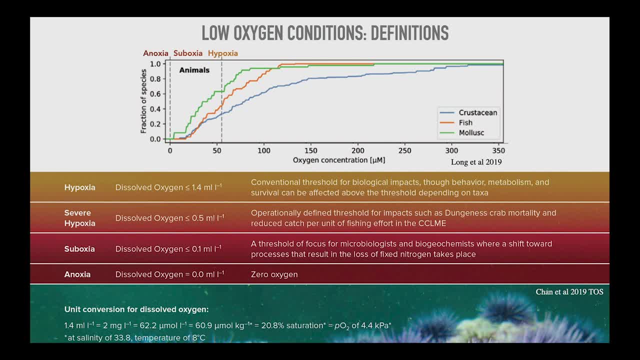 the 60 micromole, or the hypoxic boundary that we picked here, And you can see that it's about less than 50 or 40 or 60% of species can live in those thresholds. There's other thresholds that oceanographers use, like suboxia, and this is where oxygen gets really close to zero. 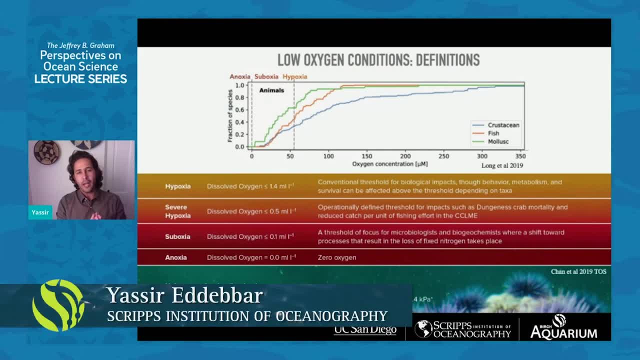 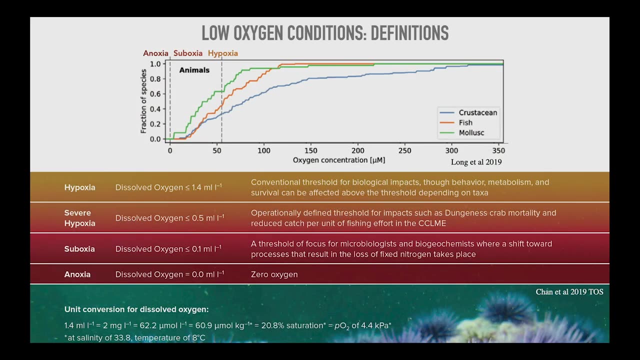 but not necessarily zero. Now that threshold, microbes begin to conduct various biogeochemical reactions that drive various changes in the nutrient cycle. We'll talk about that in a little bit. And then, finally, last term terminology that I want to define is anoxia. This is when there's no oxygen. 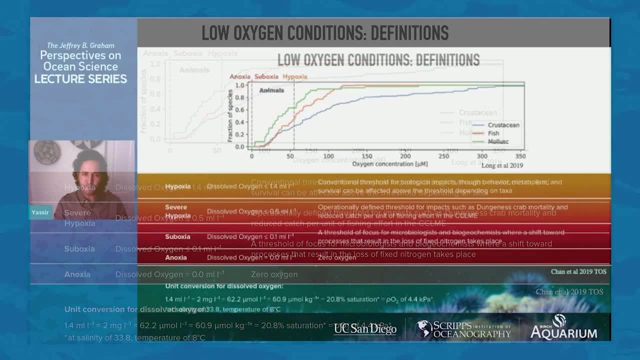 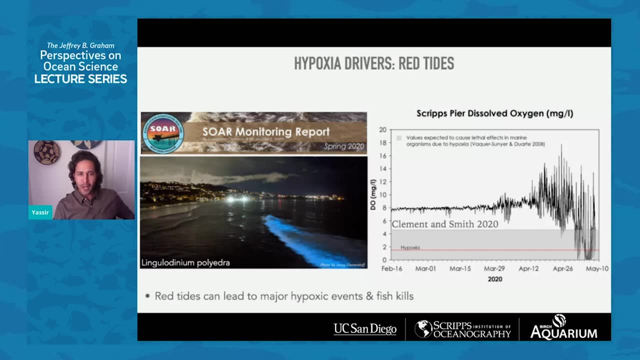 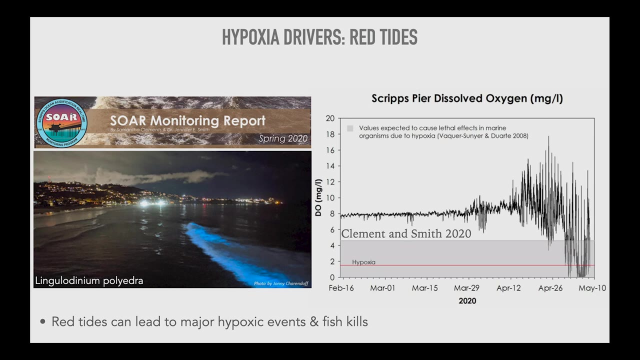 and that's also possible to be found in the ocean's interior. So we've. for many of you who are reaching us from San Diego, you've probably remembered the beautiful bioluminescence that came about in late April, in mid-late April, and then started to go away in the first couple of weeks of May. 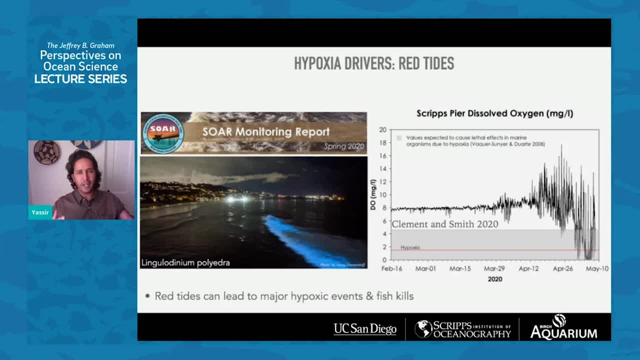 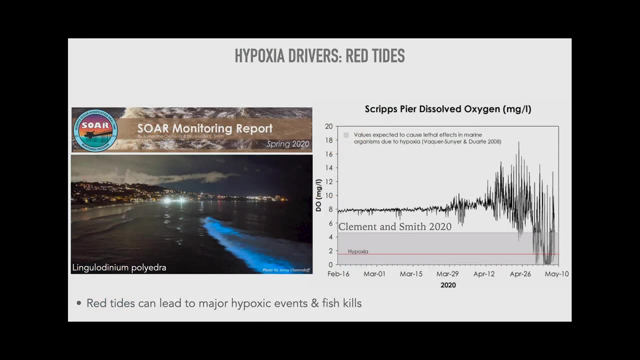 And if you live by the ocean, you would smell that stagnant smell of organic matter decomposing. And one consequence of these red tide is hypoxia. They induce hypoxic events along our coast And there's a really great lecture by Michael Latz. 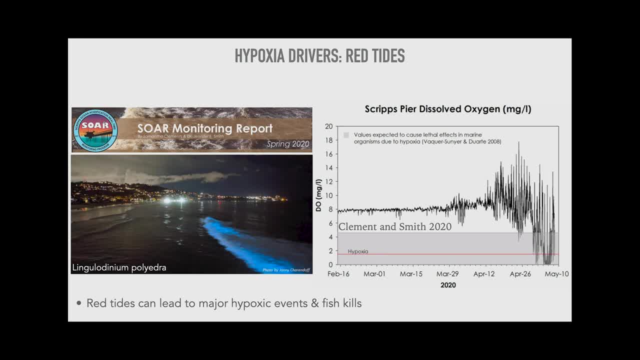 from this series that goes into the details of what red tides are, And you can see here in this time series by Clements and Smith that oxygen levels have dropped to nearly a million degrees per second And that's a really, really, really, really, really really. 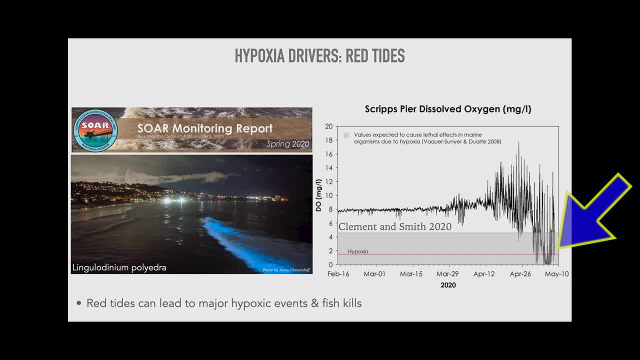 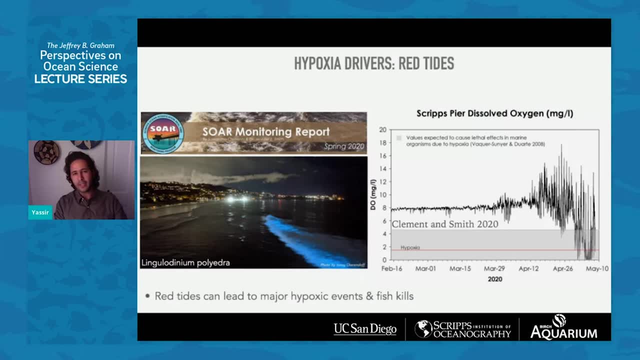 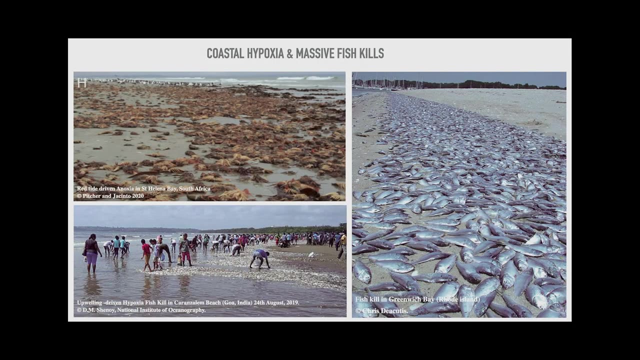 very hypoxic and also very hypoxic conditions And we've seen some fish kills occasionally here along our coast that accompanied these hypoxic events And that's really why we study oxygen, because oxygen can go down to nearly lethal conditions without any warning And that can 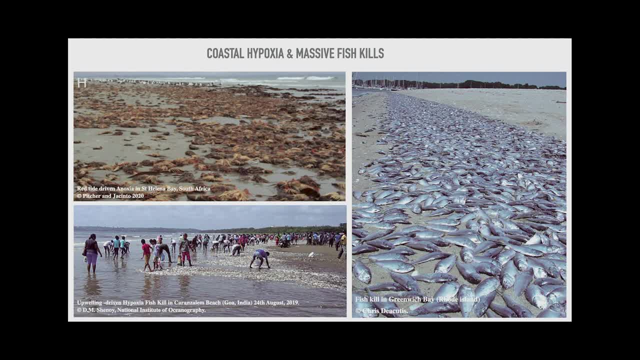 happen, for example, from coastal hypoxic events, for example from the red tides also seen here in St Helena Bay in South Africa, From upwelling driven events, for example here off the coast of Goa, India, And also from 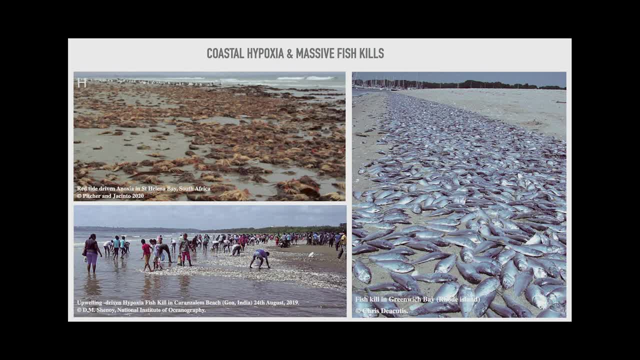 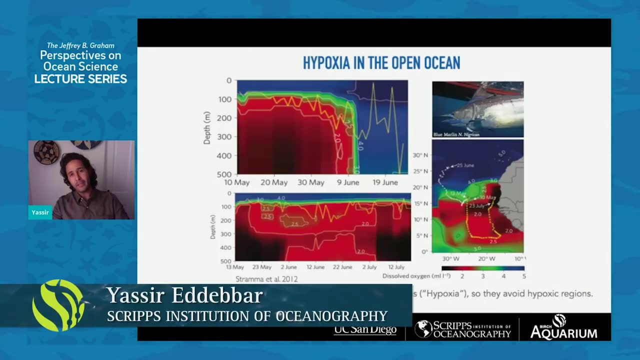 anthropogenic activities like nitrogen deposition from a wastewater treatment plant, for example, shown here from a treatment plant off the coast of Rhode Island. But what we're going to talk about today is not coastal hypoxia, but we're going to talk about hypoxia in the open ocean And to show 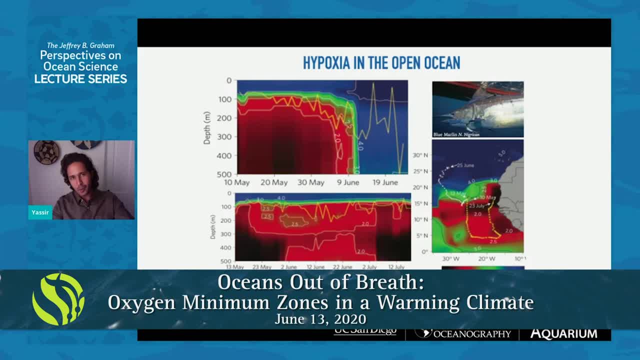 just why we want to talk about hypoxia. we're going to talk about hypoxia in the open ocean. We're going to talk about hypoxia in the open ocean. And if you want to understand how oxygen differs both in the oceans interior, throughout the open ocean, I've picked this really nice. 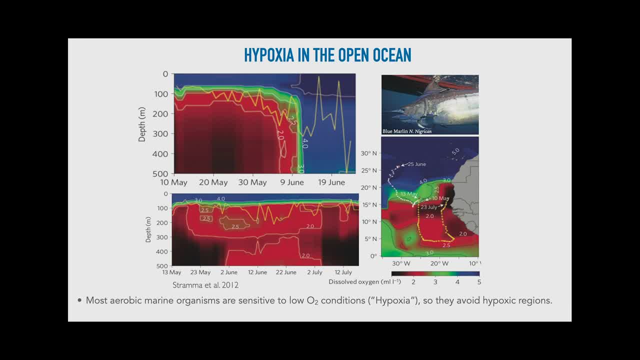 paper by Strauma, Lothar Strauma and colleagues where they tagged some blue marlins and they followed them as they got out of the oxygen minimum zone off the coast of West Africa. You can see the white line is a trajectory of the first blue marlin and it just stays in the 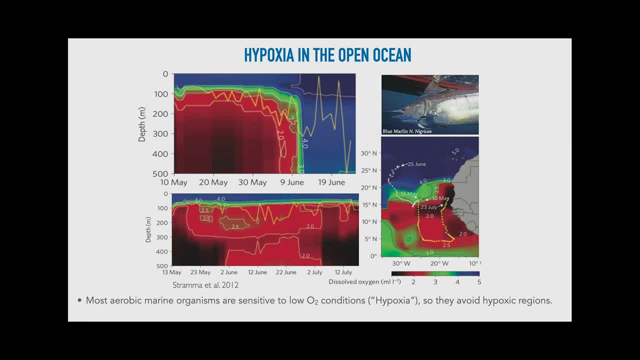 upper hundred meters, as it's over the low end of the ocean, and it's the upper 100 meters above the low end of the ocean, over the low oxygen minimum zone of West Africa, And then, as soon as it leaves, it begins to go up and down all the way from the surface. 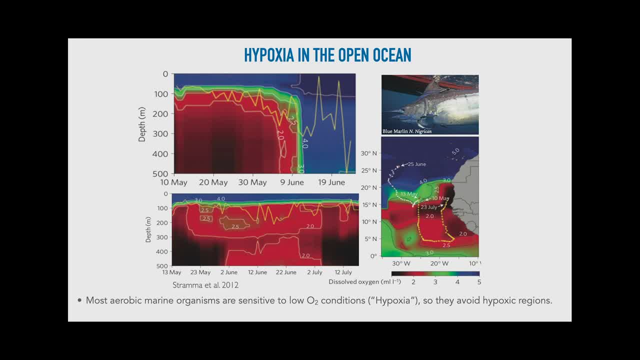 down to about 500 meters and it's able to forage without any restrictions. The other blue marlin, which stays in the oxygen minimum zone, stays largely in the upper 100 meter to 200 meters, So it's not able to go below that level of two. 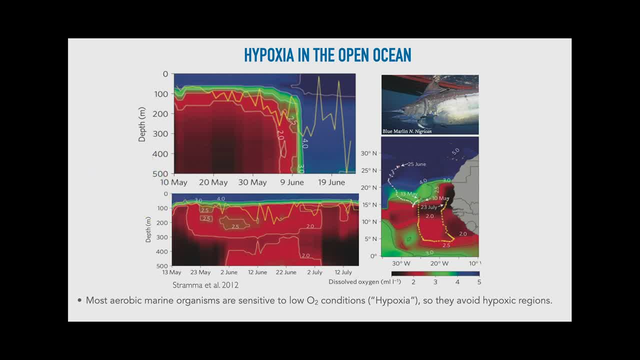 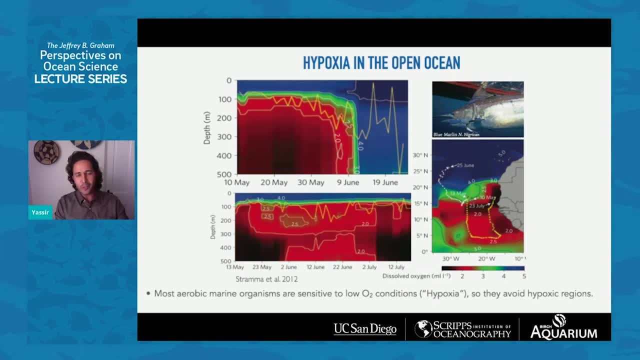 which is hypoxic and it doesn't allow it to metabolize as well. So that's really why we study oxygen in the ocean. It's extremely important to marine organism and we wanna know: why does it look the way it does in the ocean? what causes this distribution? 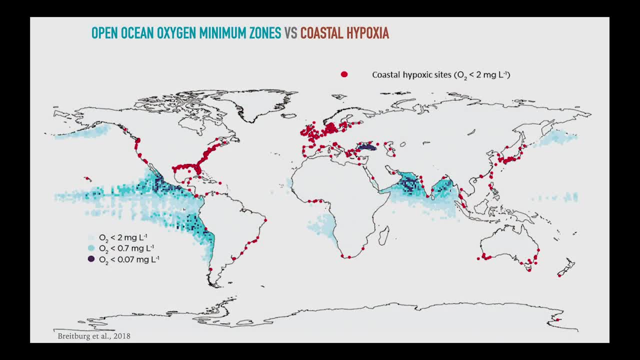 and how it's gonna change in the future. I think we have to make again the distinction between oxygen minimum zones and coastal hypoxia. So oxygen minimum zones is what you see here in blue. These are large open ocean, big areas of oxygen minimum. 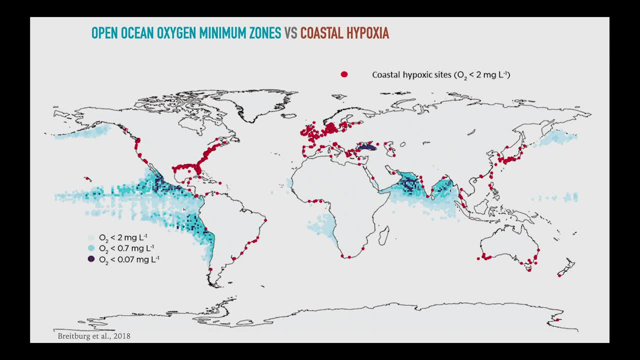 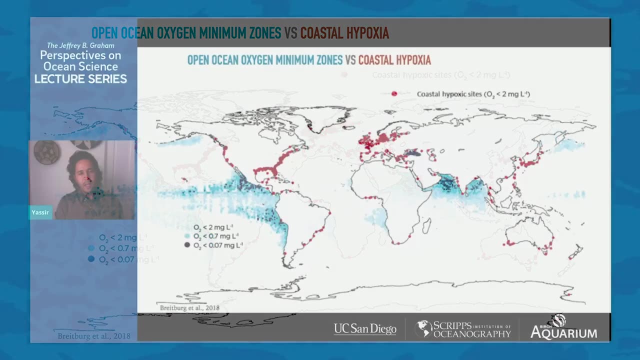 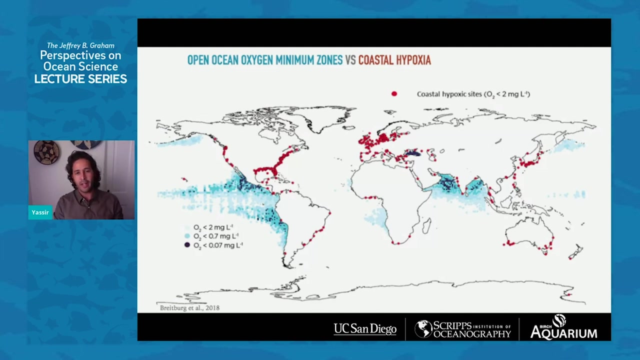 that occur naturally, and we'll talk about what's driving them, whereas hypoxic coastal regions are constrained to the coastline and they're typically either driven by natural phenomena like red tides, but also anthropogenic effects like the delivery of nutrients from wastewater treatment plants or agricultural activities. 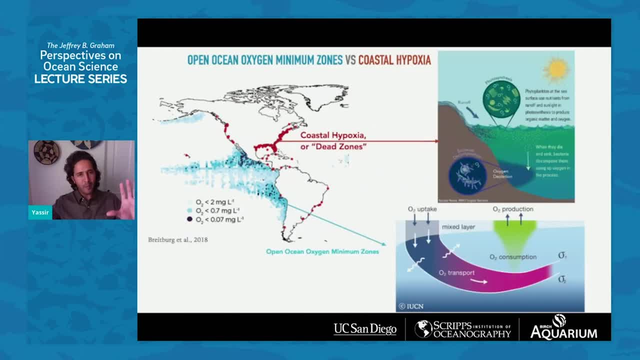 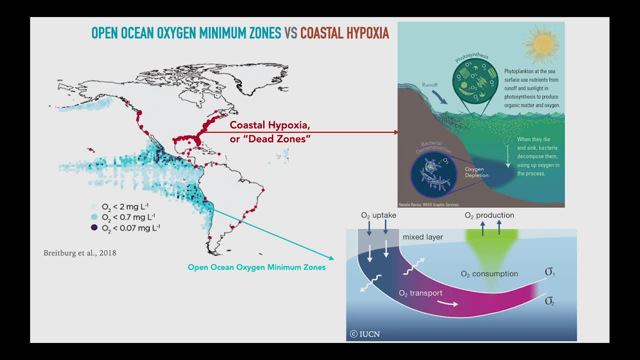 So it's really important that we separate these two phenomena because they get confused a lot in the public's mind. So the first one: coastal hypoxia, or you've probably heard of them as dead zones. they result from this process called eutrophication. 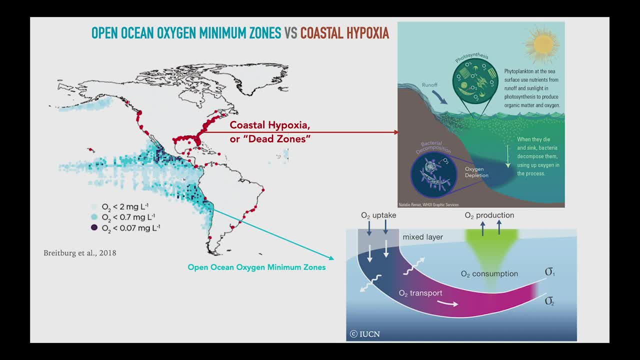 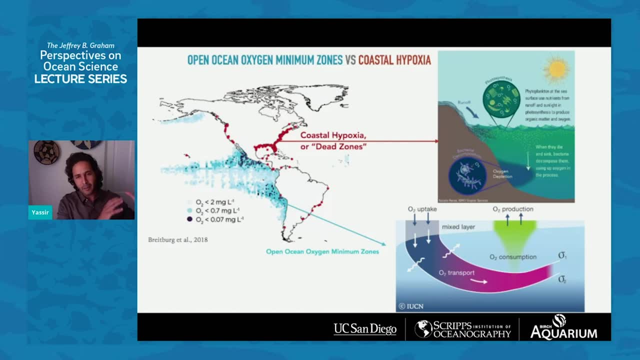 So say, there's an agricultural field or bar-scale industrial processes along the coast, for example off the east coast of the United States, and there's a massive rain event and that rain event drags all the nutrients, nitrogen and all the pollutants out. 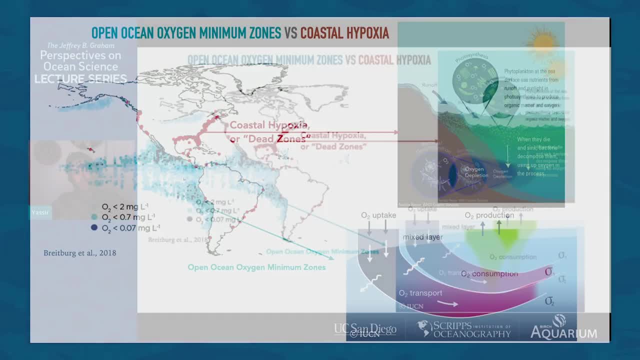 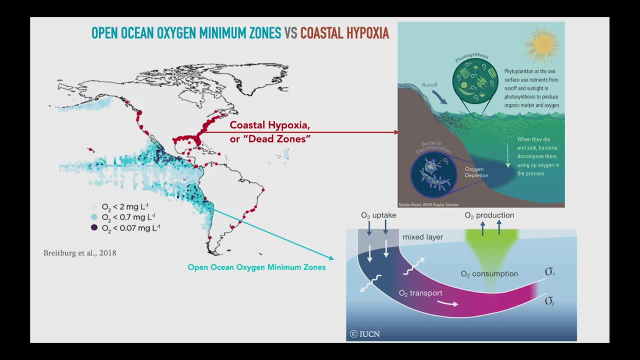 offshore that fertilizes the upper ocean, And all that fertilized phytoplankton that grows ends up deposed in the ocean's interior, along the coast, and decomposes, And as it's decomposing, microbial organisms remove oxygen and we end up with these oxygen-dead zones along the coast. 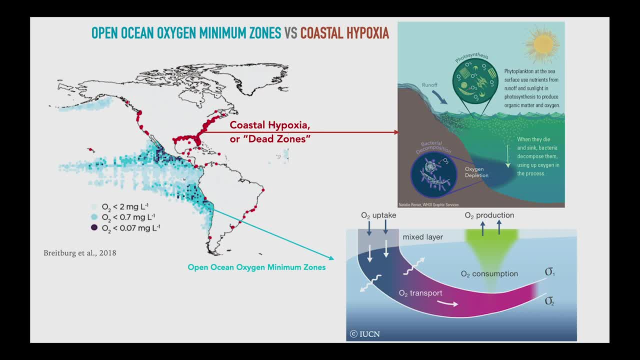 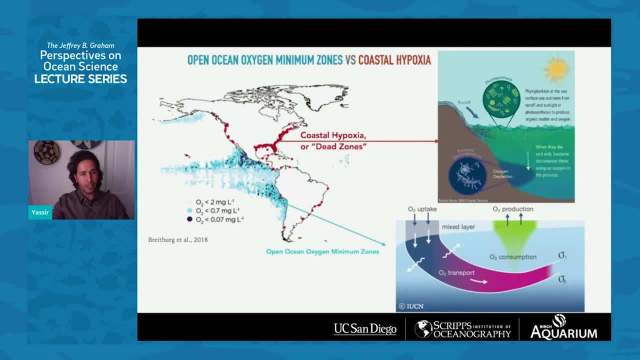 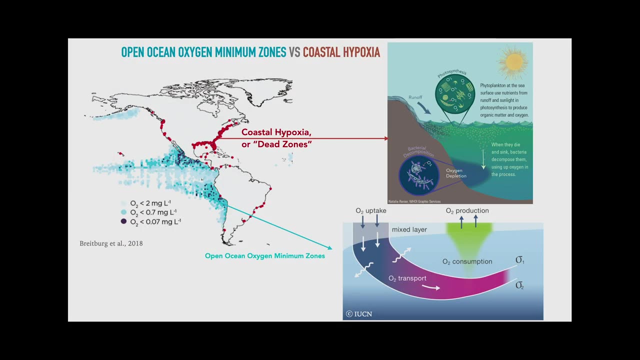 The oxygen minimum zones that we find, for example, here off the tropical Pacific. these are related to microbial consumption and production from the open ocean, but they're also associated with the large-scale circulation of the ocean. There's a component which we call ventilation: how much water circulation is happening in that region? 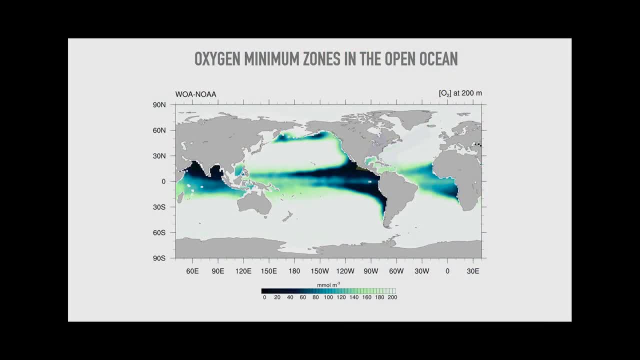 So where can we find oxygen minimum zones? So we can find the biggest ones, for example, off the northern tropical Pacific. So that's one of the biggest oxygen minimum zones. So we can find the biggest ones, for example, off the northern tropical Pacific. 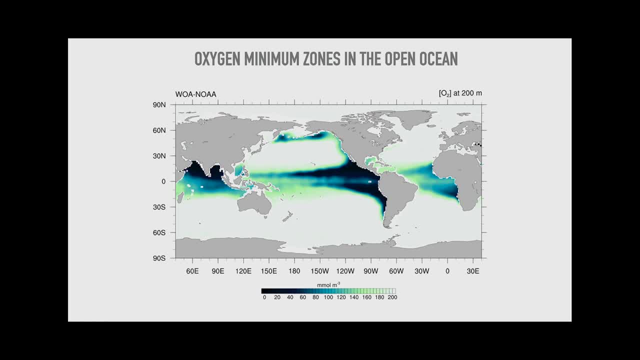 So that's one of the biggest oxygen minimum zones, So we can find the biggest ones, for example- and you can see it here- with values below 60 millimol per meter cube. There's also another one south of it. This is the south tropical Pacific OMZ, And then in the northern tropical. 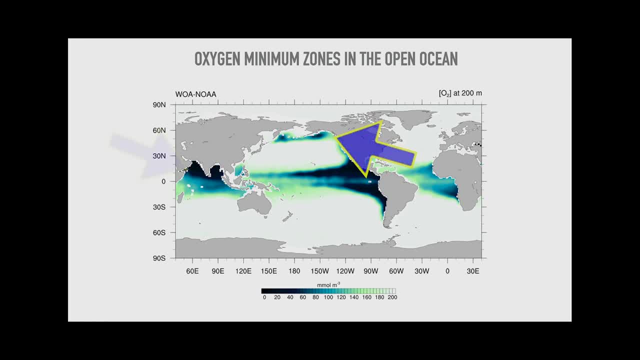 Pacific, there's another one called the north tropical Pacific OMZ, And then, off the coast of India, in the Indian Ocean, the Arabian Sea, there's a very intense oxygen minimum zone that extends pretty far south, And then finally, in the Atlantic, there's a couple other oxygen minimum. 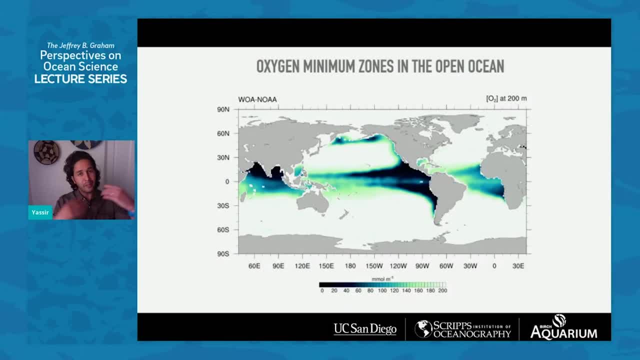 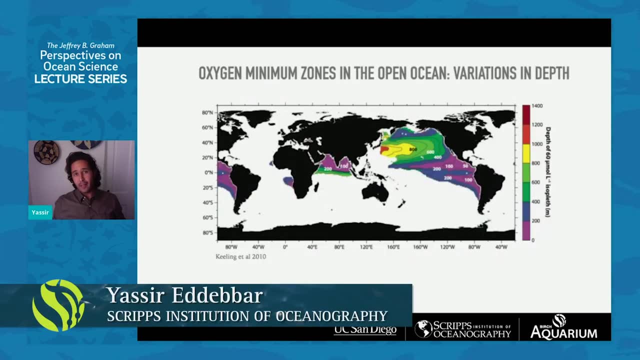 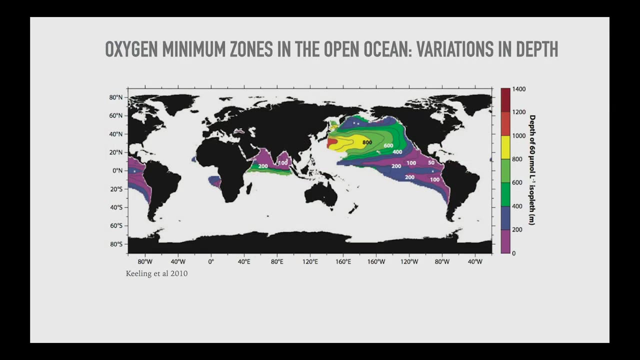 zones, but they're fairly weak, And that's as we're going to see, because there's a lot of ventilation in the Atlantic. So these oxygen zones are really fascinating. They have very different character. Each one differs, So there is, for example, a lot of variability between them. just 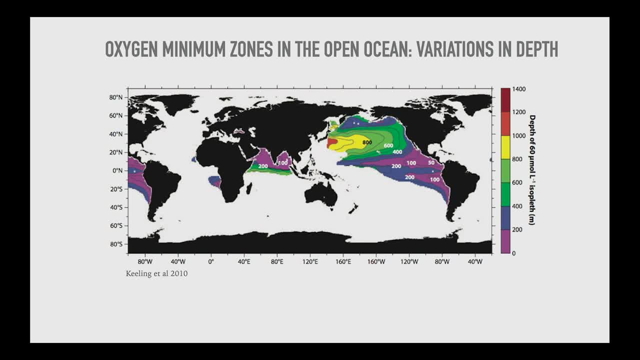 in the depth. So if you go to the tropical Pacific OMZs you're going to reach hypoxic depth at about 50 to 100 meter depth. So off the coast of India, you're going to reach hypoxic depth. If you go to the Gulf of Costa Rica or Mexico, if you were to go offshore, you can find. 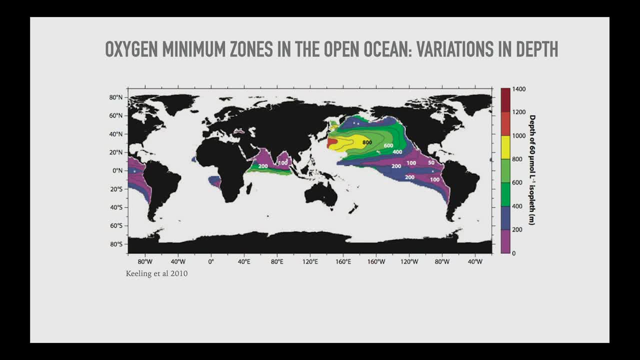 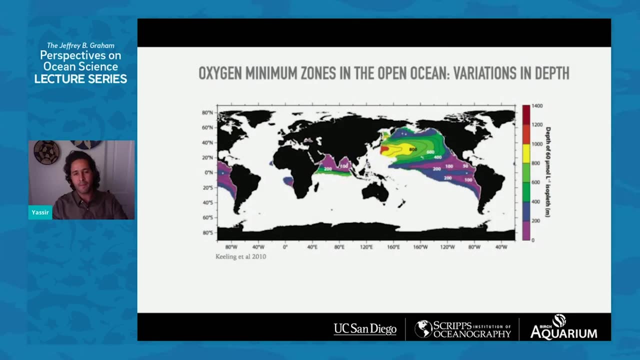 an oxygen minimum zone there, just in the upper 100 meters, Whereas the oxygen minimum zones of the Atlantic are going to be deeper And you're also going to see much deeper oxygen zones on in the northern Pacific. That reflects again this process of ventilation. So why are the oxygen? 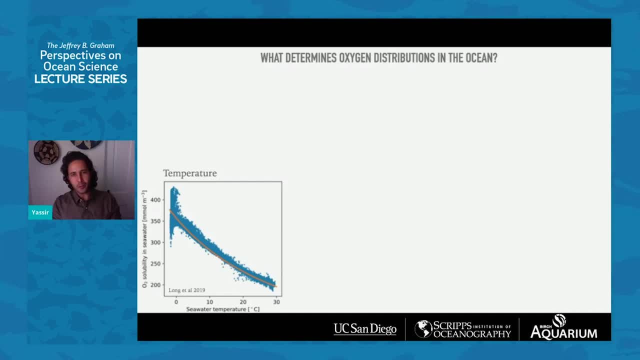 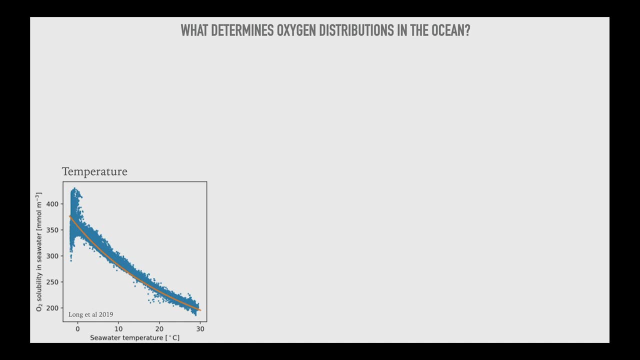 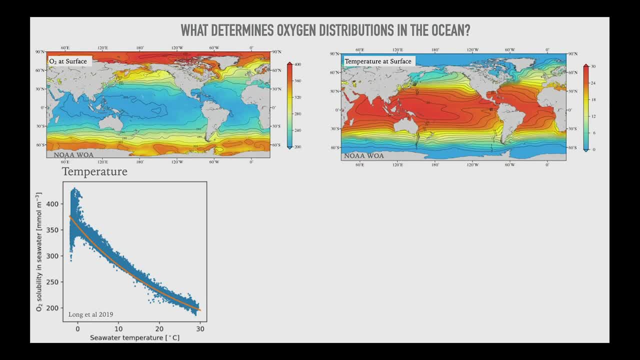 solubility in seawater decreases And you can actually see this in the upper distribution of oxygen at the surface. So we know that the low latitudes are usually warmer. They receive more sunlight than the high latitudes And as a result, there's less oxygen at the surface in low latitude versus the high latitudes. So 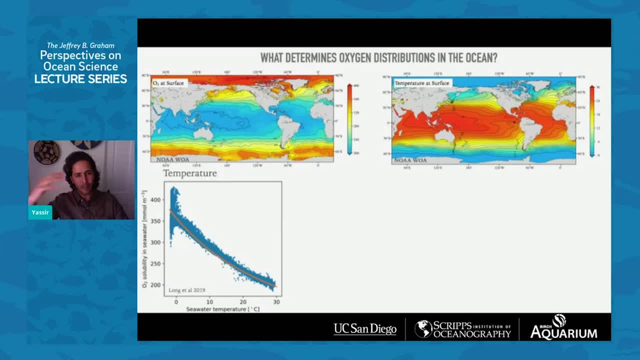 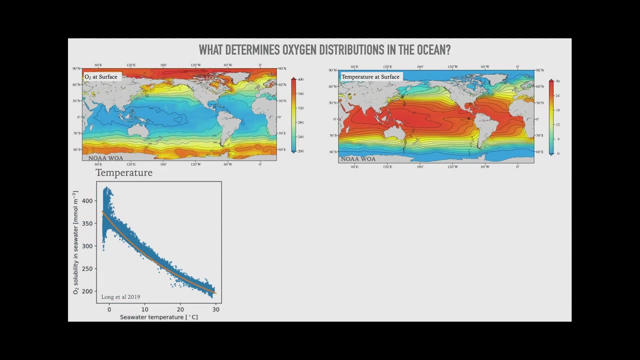 that's the number one process at the surface that's operating in the mixed layer. Also, there's a lot of exchange between the mixed layer, the upper part of the ocean and the atmosphere, at all times between these two elements, And so whenever there's an undersaturation or less oxygen at the 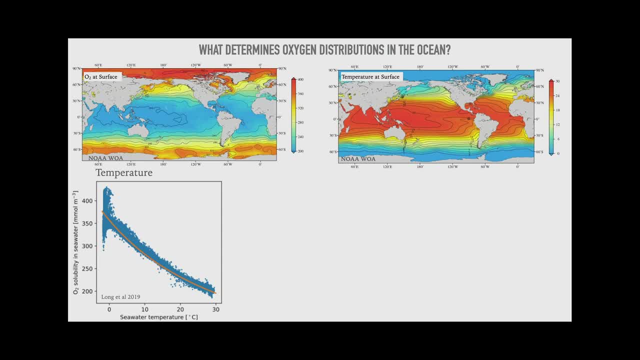 surface, the mixed layer is able to run, And so that's the number one process at the surface And that's the number one process at the surface And that's the number one reason why we're able to absorb that oxygen right away from the atmosphere. However, if you go down to 200-meter depth, 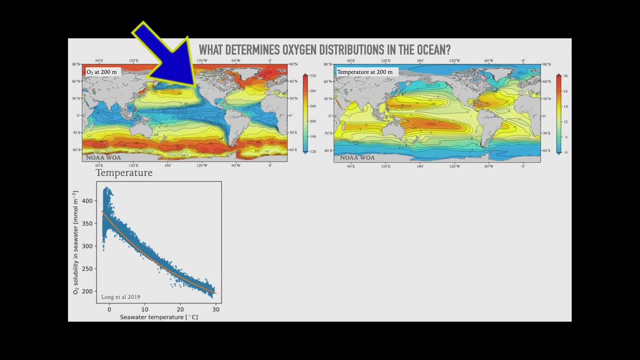 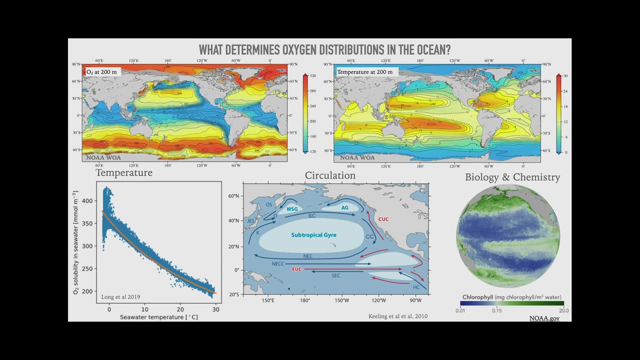 you're going to see a slightly different pattern. You're going to see this pattern where there's low oxygen along the eastern part of the basins here off the Pacific and the Atlantic and the Indian Ocean, And that's not necessarily related to the distribution in temperature. So that's where the 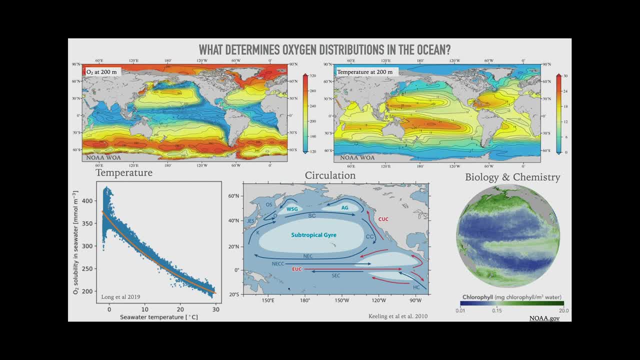 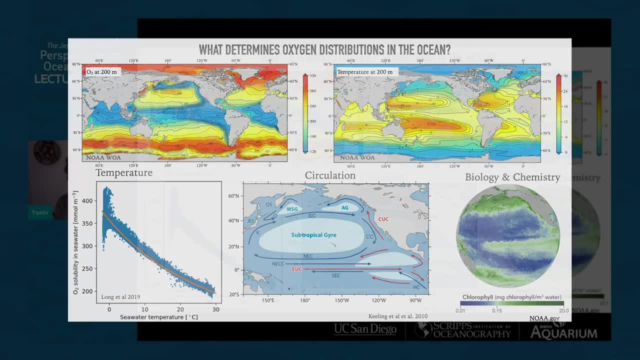 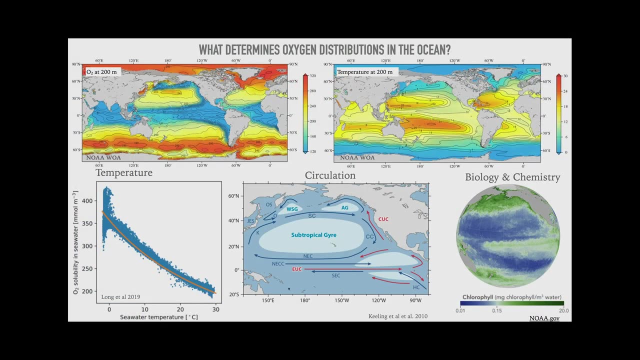 effects of circulation and biology and chemistry come into play. Now in the open ocean there is what we call the subtropical gyre. Many of you are familiar with subtropical gyres here, with the Great Pacific Garbage Patch, for instance, And what you'll notice. 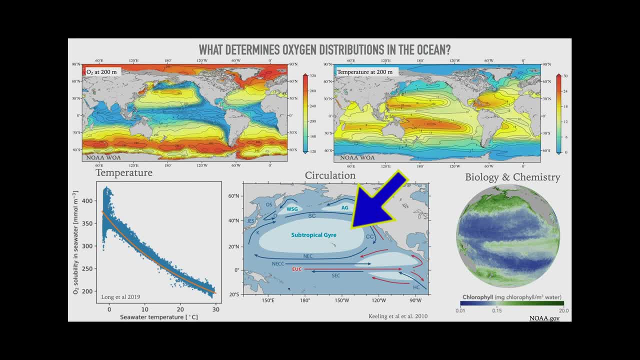 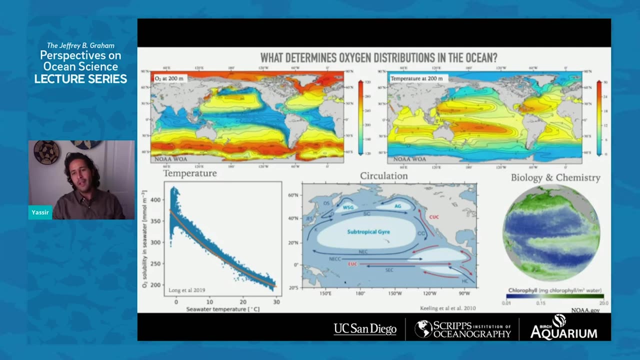 is that the subtropical Pacific gyre and its anticyclonic flow essentially misses the eastern part of the Pacific, So that's what we call the shadow zones. So there's just not enough ventilation, not enough oxygen. is that part of the ocean? And the other part of this process is biology and chemistry. What you 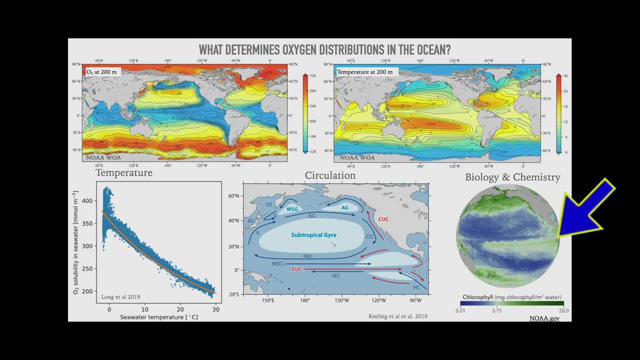 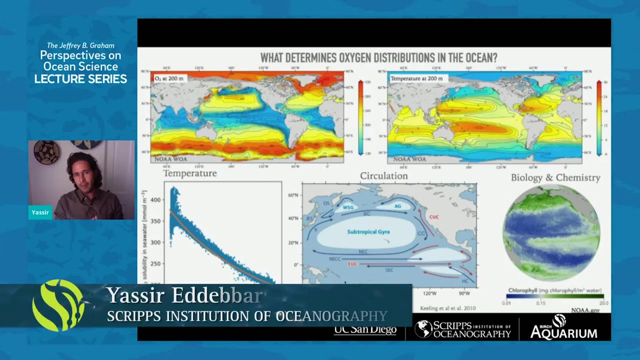 notice is that along the equator there's a lot of upwelling, There's a lot of biological activity and phytoplankton at the surface. That phytoplankton again sinks, similar to what we see here with coastal hypoxic events, And as it's sinking, microbes are able to. 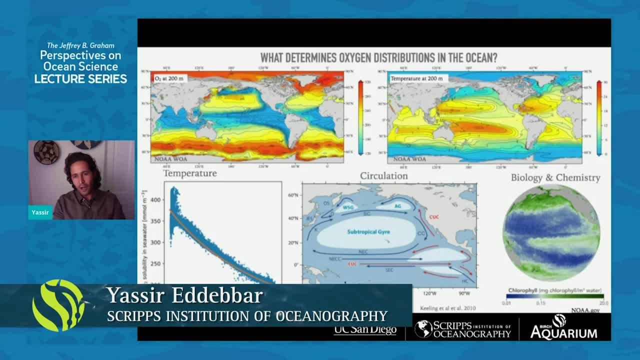 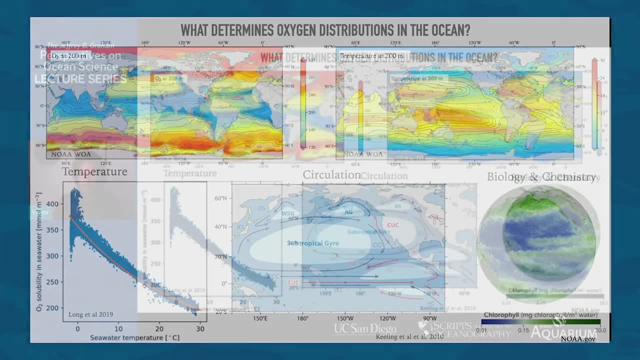 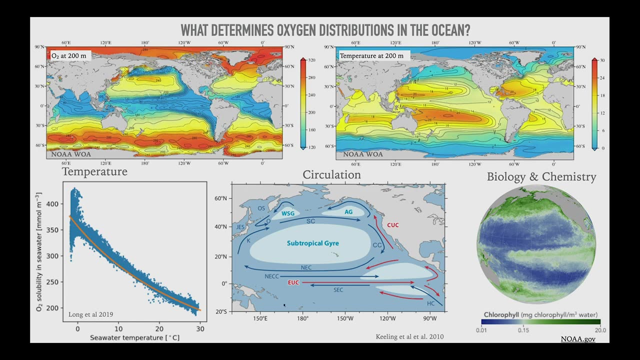 respire all that organic matter. So they remove oxygen and they remodelize it into CO2 and nutrients, And so the balance of oxygen, essentially this balance between circulation and biology, at depth, with some contributions from temperature, but at the surface it's mostly. 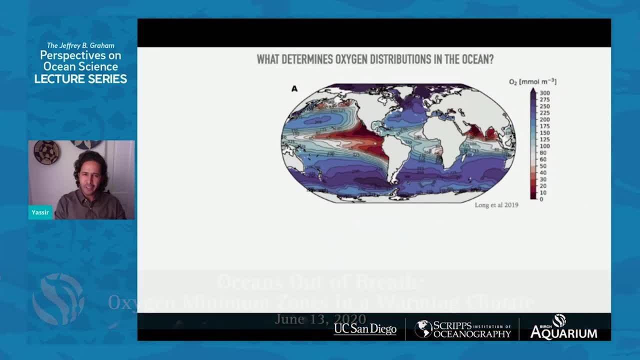 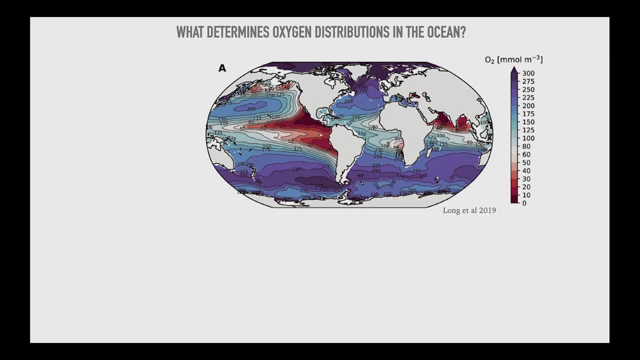 distribution of oxygen at 150 meter depth And you can again see the oxygen minimum zones in red. And when I superimpose the subtropical gyres circulation, you can see that they essentially the regions where they are not reaching. the basin is where you're going to. 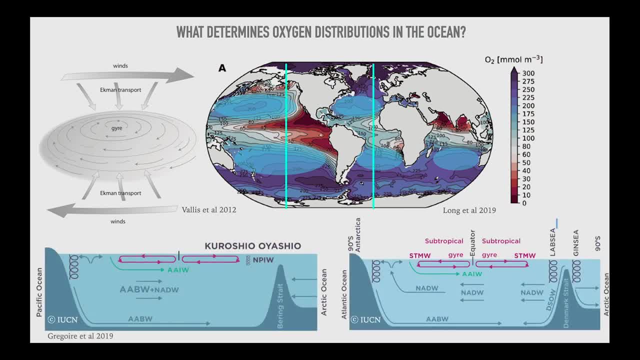 find these low oxygen minimum zones. If you were to take a transect right through the Pacific and the Atlantic, you're going to see differences in that ventilation. you will also see differences in how much oxygen reaches the oceans interior because of what we call the overturning circulation. 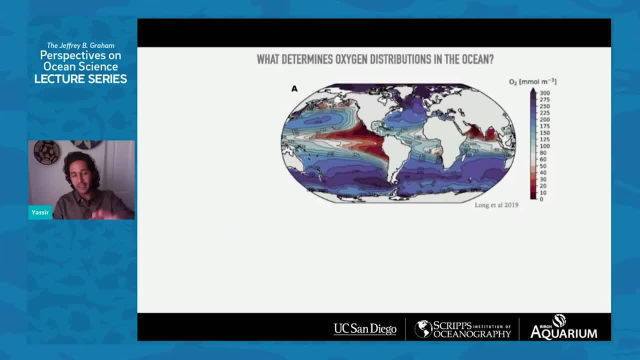 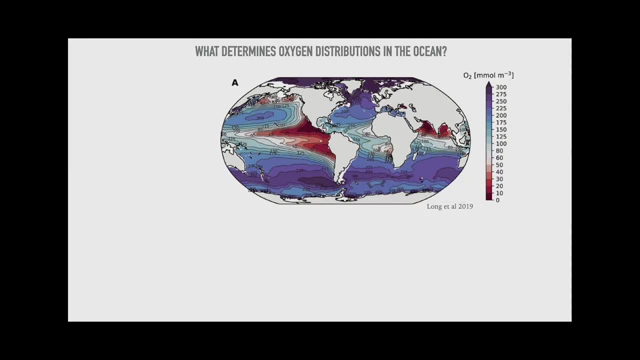 And that's really important to try to understand differences between the Pacific and the Atlantic, for example, the Pacific has much bigger oxygen minimum zones, largely because there's not enough overturning circulation, not enough deep water that forms in the North Pacific and the Atlantic. 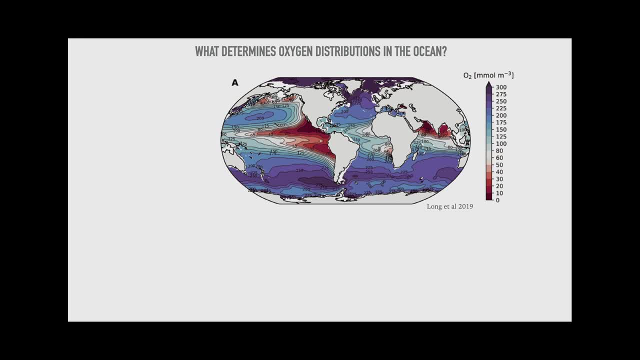 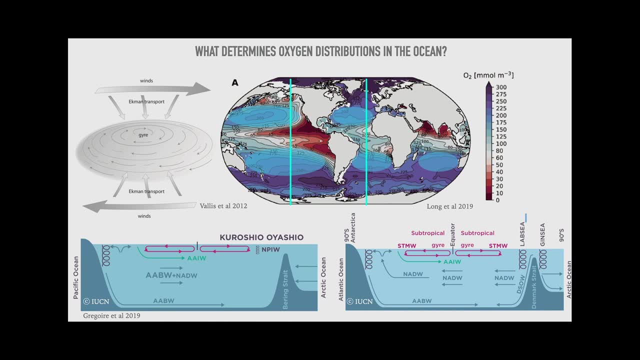 And ventilates the oceans interior, whereas the Atlantic. there's a lot of oxygen ventilation from North Atlantic deep waters. So this is water that forms here off the coast of Greenland in Canada and descends and on its descent it ventilates the rest of the interior. So think of the oxygen. 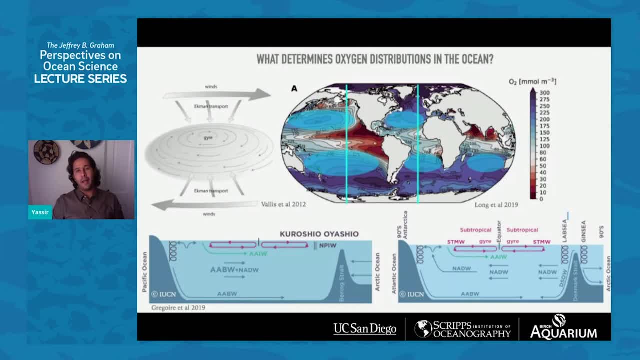 minimum zones, as your basements at home, And the high latitude and mid-latitudes are the windows to your home, So you can see that there's a lot of oxygen in the deep waters of the Atlantic. because the basement is so far away from these windows, they don't get enough circulation and 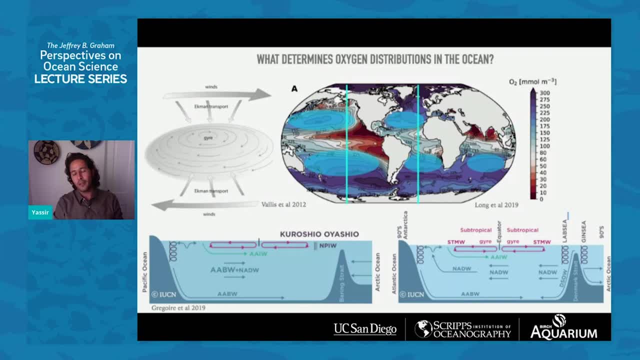 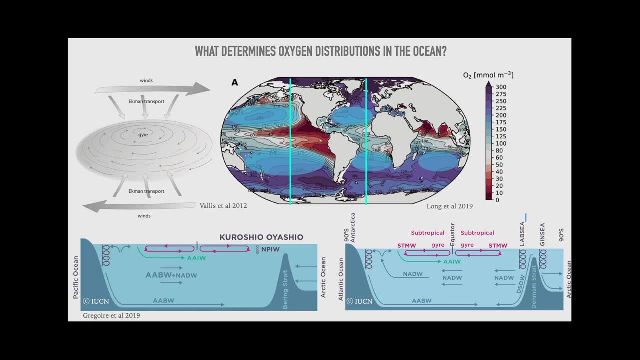 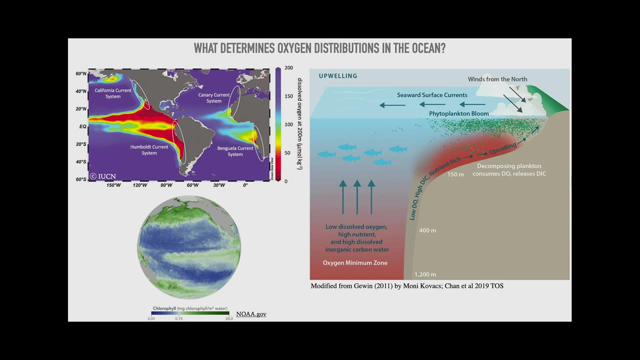 they're going to feel stagnant and the air there is going to feel old. And so, the same way that ventilation occurs in your home, it's essentially the same process here in the ocean. there's just not enough ventilation reaching that area. But there's other processes. for example, 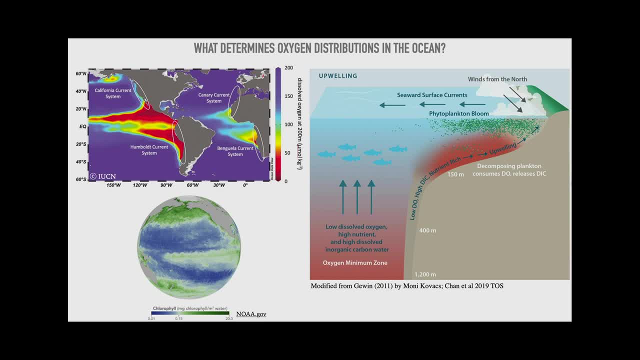 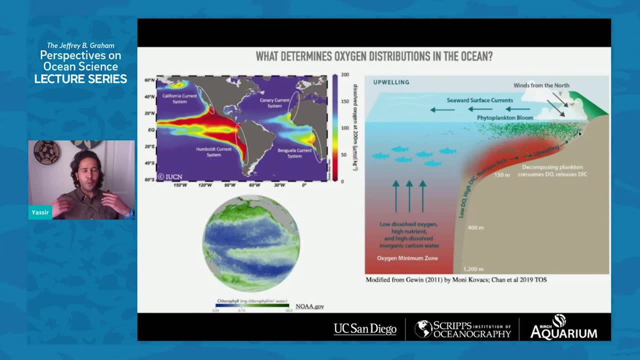 the oxygen minimum zone off our coast here in the California current region is driven in part by upwelling. So during spring, for example, you notice that there's more winds coming from the northwest, And those winds are driven in part by the temperature difference. 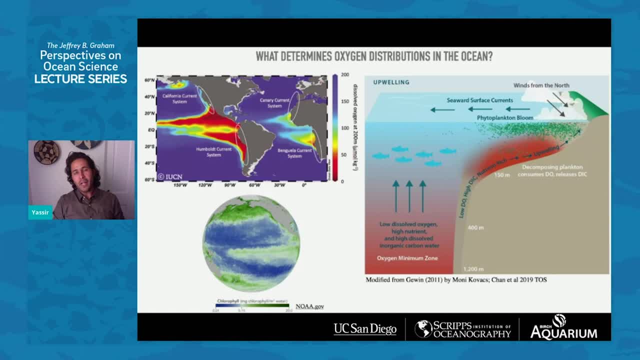 between land and ocean. Land just warms much faster than the ocean. that creates a gradient in pressure and it creates winds that go towards the equator. Those winds push water not with them towards the equator but to the north of the equator. So you can see that there's a lot of oxygen. 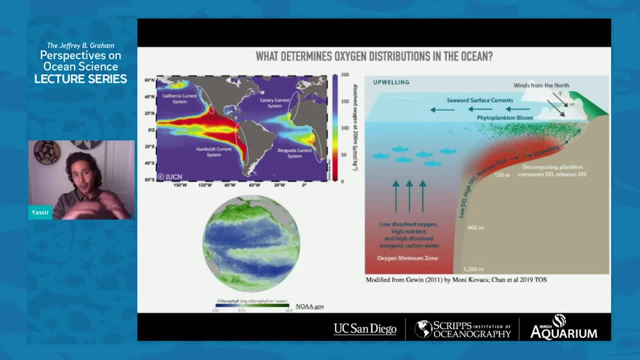 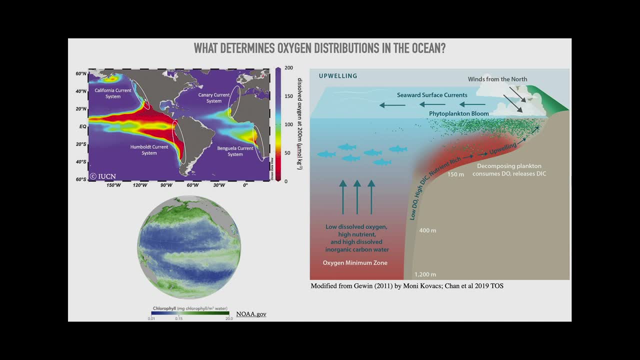 coming from the north to many degrees to the right, And that's because the Earth rotates, And so, as those waters are being pushed offshore, upwelling brings up low oxygen water that comes up to the surface and it's filled with nutrients and that's going to fertilize the surface. For 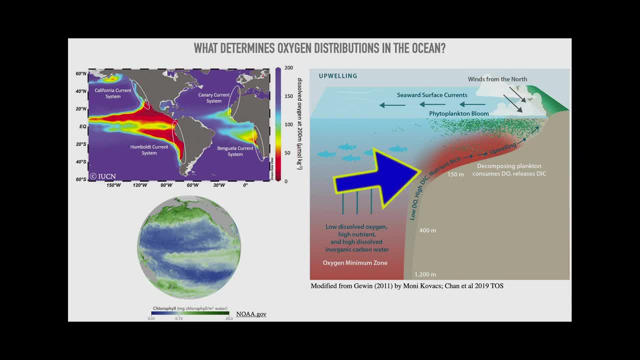 example here, as we can see, low dissolved oxygen, high carbon, water that's rich in nutrients comes up to the surface and fertilizes the surface, And then again, as that phytoplankton bloom begins to grow, it's going to start to grow, And then again, as the phytoplankton bloom begins, 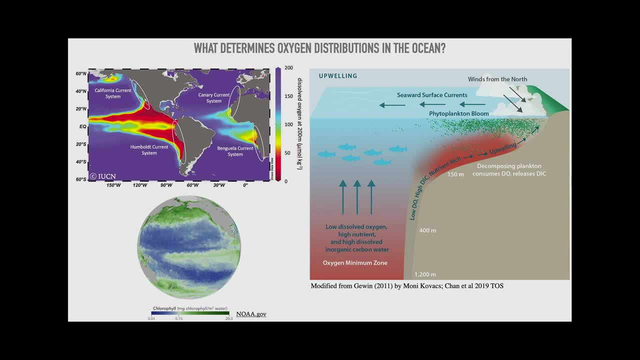 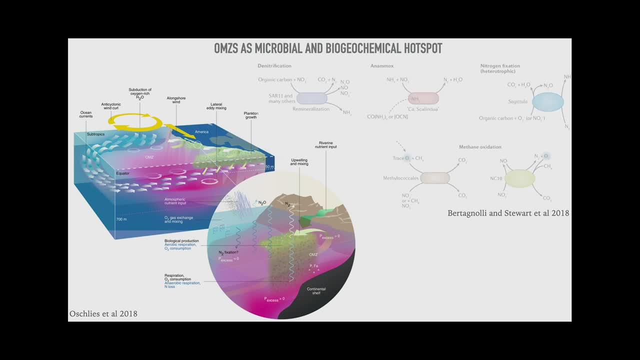 to grow. it's going to start to grow, And then again, as the phytoplankton bloom begins to grow, it's going to start to grow, And then again, as the phytoplankton bloom begins to die and descend into the ocean's interior, microbes begin to respire, And that's really sort of what's. 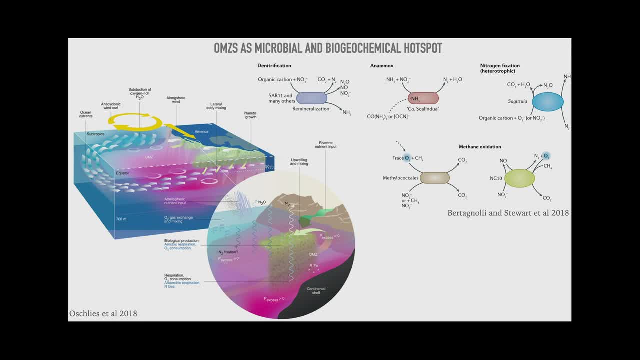 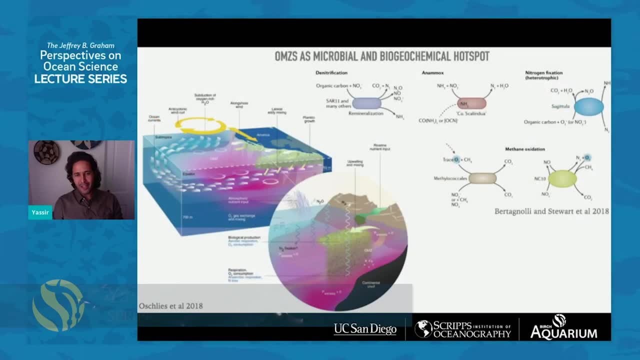 driving the existence of the oxygen minimum zones, And we can go more and more about all the details of the oxygen minimum zone. I think that's what I find really fascinating about these phenomena is that the more you dive in, the more you realize that they're extremely fascinating, extremely. 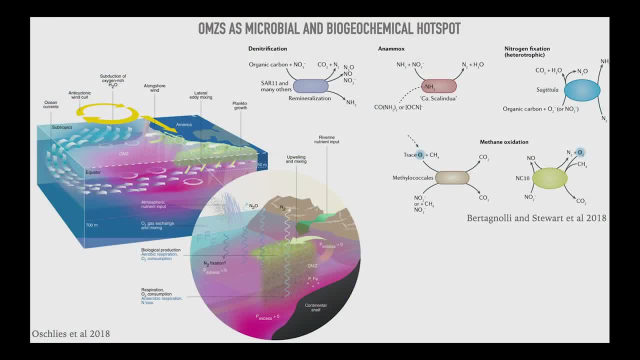 complex with all kinds of phenomena, And I think that's what I find really fascinating about these phenomena is that the more you dive in, the more you realize that they're extremely fascinating with feedbacks, And this is one example. Here's some of the processes from the most recent literature. 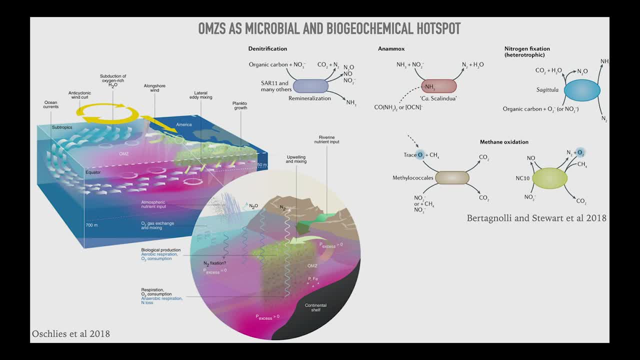 that shows the oxygen zone, for example off the northern eastern tropical Pacific. It includes contributions from ocean circulation. And within the oxygen zone itself there's a variety of microbial processes that remove nutrients or recycle nutrients, for example the process of denitrification. And then within the oxygen zone itself there's a variety of microbial processes that remove nutrients or recycle nutrients, for example the process of denitrification. And then, within the oxygen zone itself, there's a variety of microbial processes that remove nutrients or recycle nutrients, for example, the process of denitrification. And then, within the oxygen zone itself, there's a variety of microbial processes that remove nutrients or recycle nutrients, for example, the process of denitrification. 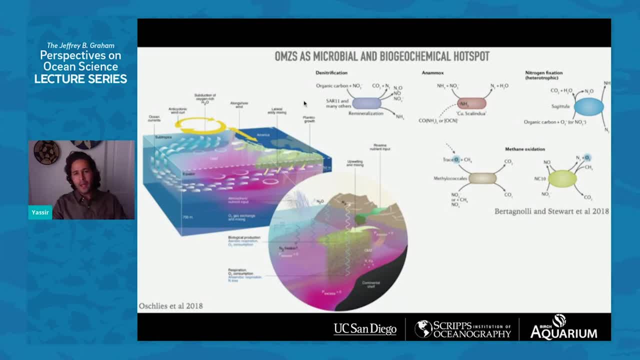 Which occurs when oxygen is much lower, And it creates nitrous oxide, which is a byproduct of this reaction and a very powerful greenhouse gas. So these are just examples of some of the chemical and biological processes that are happening in the oxygen minimum zones. 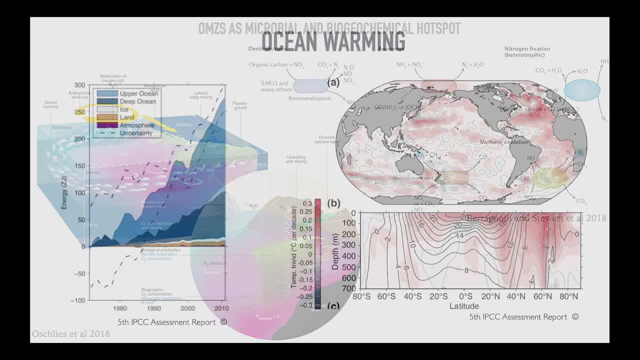 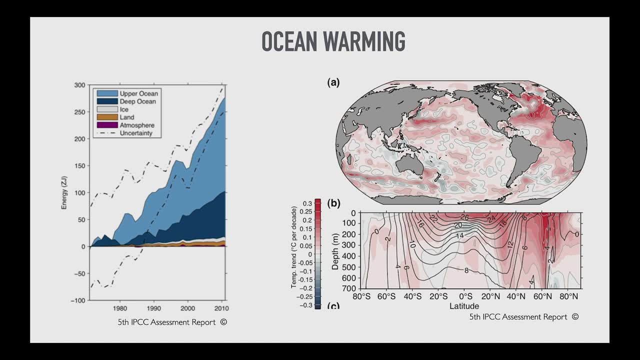 And it's important to just sort of take a step back and see how much the ocean has done in terms of mitigating climate change. So, because of the buildup of greenhouse gas in the atmosphere, most of the heat trapped by greenhouse gas emissions have gone mostly into the ocean. 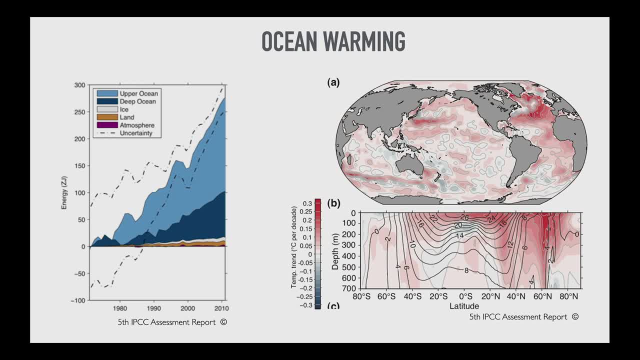 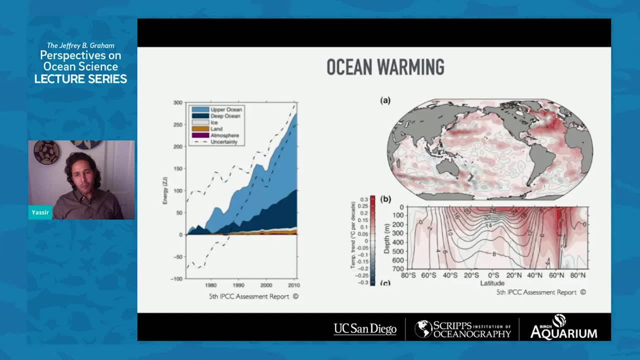 That's because the ocean is large, It's very deep, It's very dynamic, So it circulates, It's able to take that heat and put it in its interior And, very importantly, it's got a large heat capacity. It's able to absorb a lot of heat for very little temperature change. 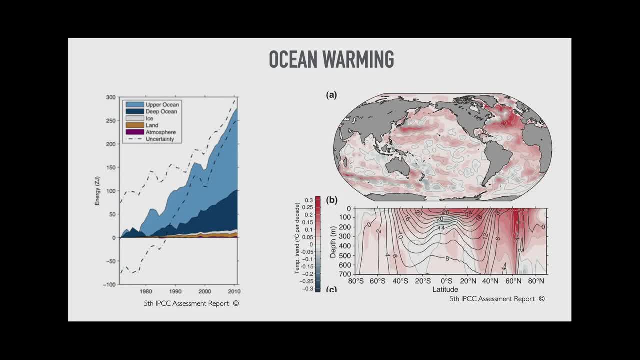 You can see it here in the panel to the left, You can see the amount of energy trapped in different parts of the planetary system And you can see that the atmosphere, land and ice only account for a small portion of the energy trapped by. 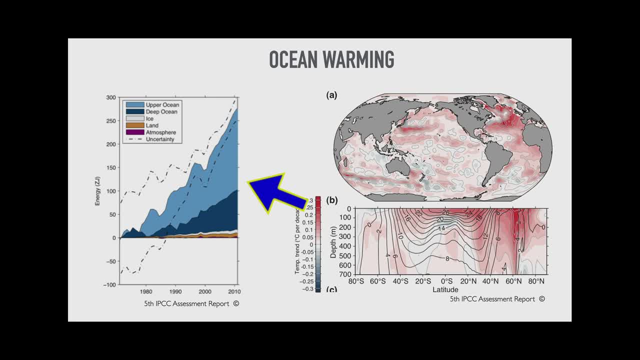 the greenhouse gas emissions, Whereas most of the heat is trapped by the ocean And a lot of it has gone into the upper ocean. So this is the upper 1,000 meter And you can see it in the distribution of ocean heat that's recorded in temperatures over the last six decades. that 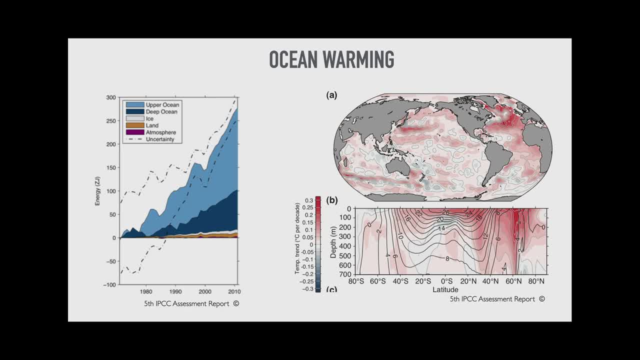 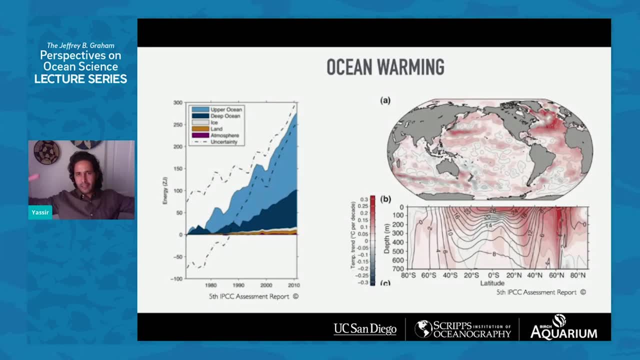 the North Atlantic, North Pacific and the Southern Ocean have warmed the most And that's because, again, they're the windows into the ocean's interior And, as the atmosphere is warming up and most of that heat is going into the ocean, it's going to go into the ocean through this mid. 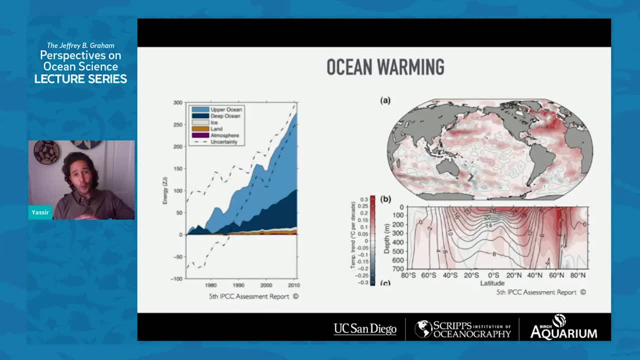 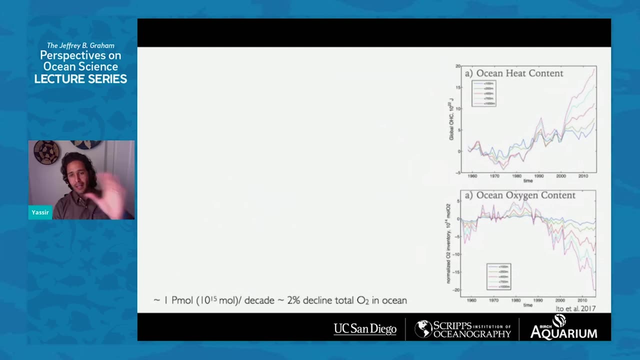 and high latitude region of ventilation. So we're going to hear more about this from Professor Sarah Gilley next. I'm really excited to hear about that. What we are interested in is how this warm impacts oxygen. So in the last five or six decades, as the ocean heat content have gone up in 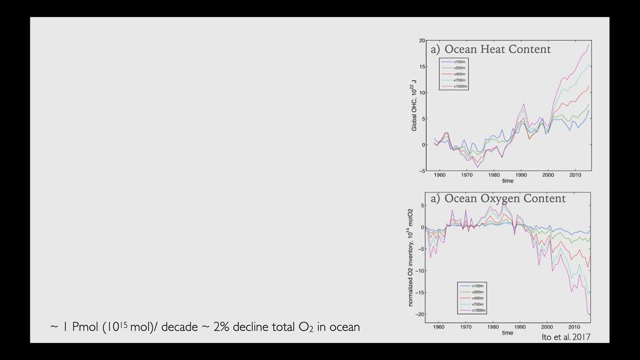 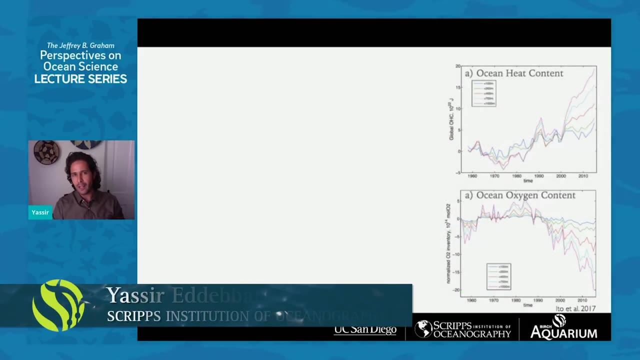 the upper 1,000 meter. we've noticed in the observations that the oxygen content globally has decreased, And that's the rate at which it decreased is about 2% of the total oxygen inventory. That might not seem like a lot, But 2% is a lot, especially for regions where oxygen is. 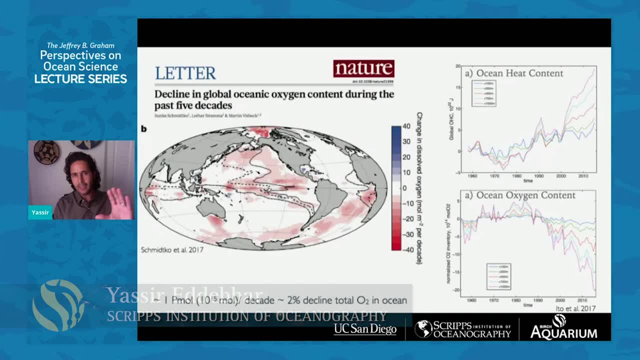 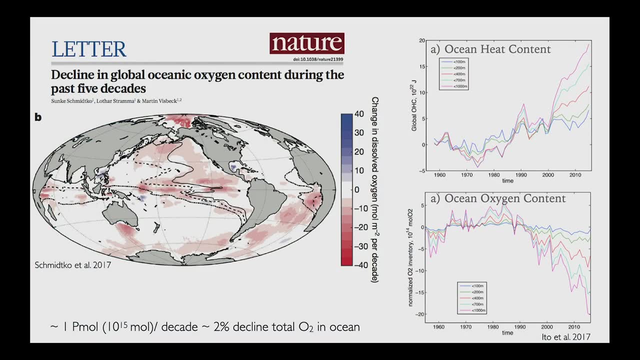 overwhelming And you can see that in the distribution of the oxygen loss that we've recorded that a lot of it is in regions, for example here in the tropical Pacific, where oxygen is already low. So the decline in oxygen in these regions where oxygen is already, 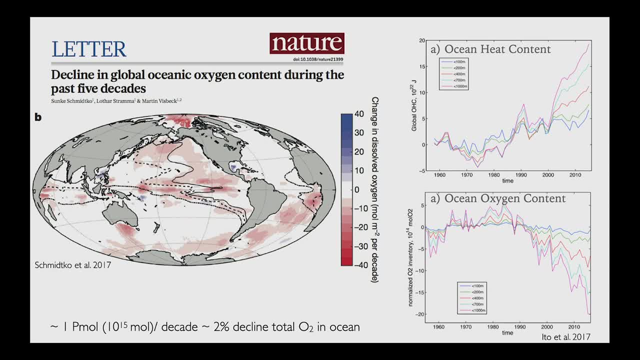 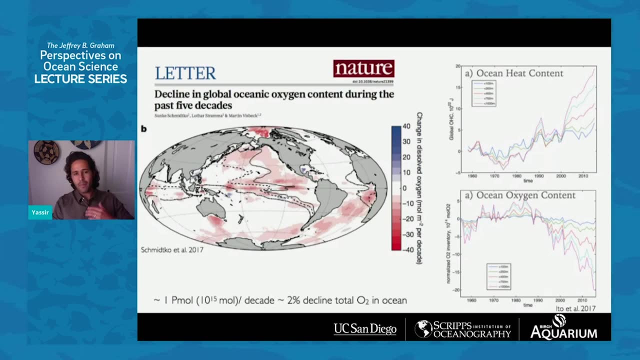 naturally low, can have a really big impact on where that hypoxic depth sits. You can also see there's a lot of changes in the Arctic, in the Southern Ocean and in the South Atlantic, And so when we say 2% decline in total oxygen in the ocean, that's really the global mean It. 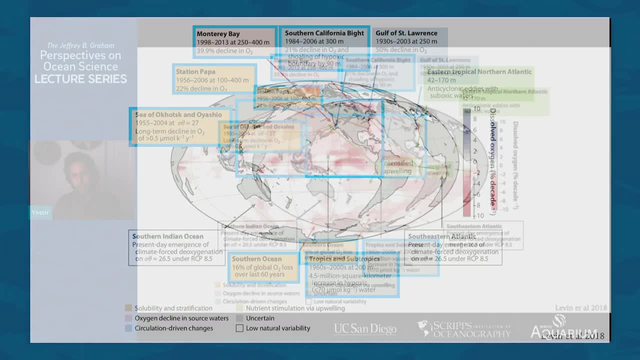 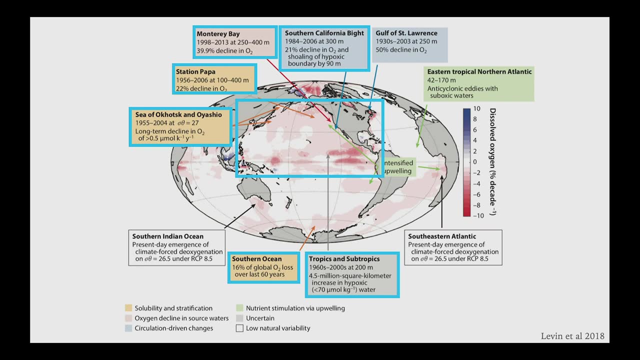 doesn't say much about the regional changes- And this paper by Professor Lisa Levin really highlights that where we can see, for example, especially in the North Pacific, that the tropics account for about 40% of that change: the tropics in the North Pacific, In certain areas like the. 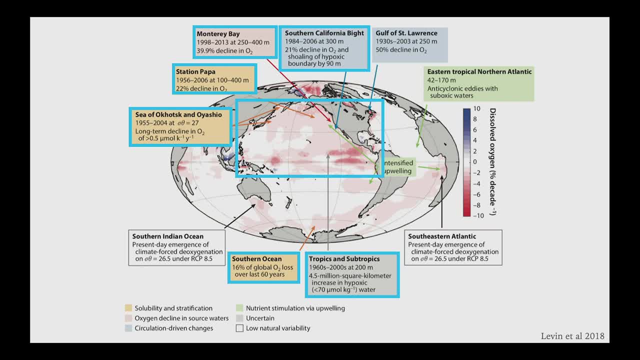 Southern California Bight, just the northern California Bight, the northern California Bight, just offshore from here. there's been a 21% decline in oxygen from 1984 to 2006 at a depth of about 300 meters In Monterey Bay. we've seen declines of about 40% In Station Papa, which is 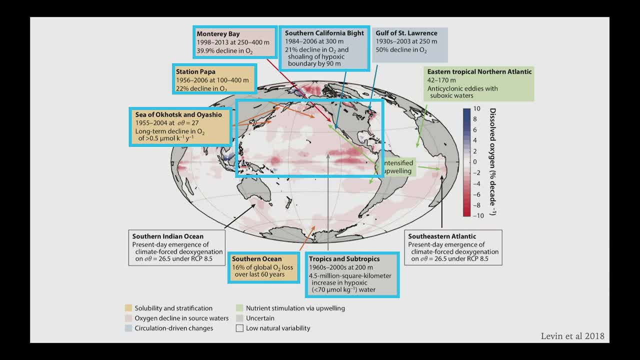 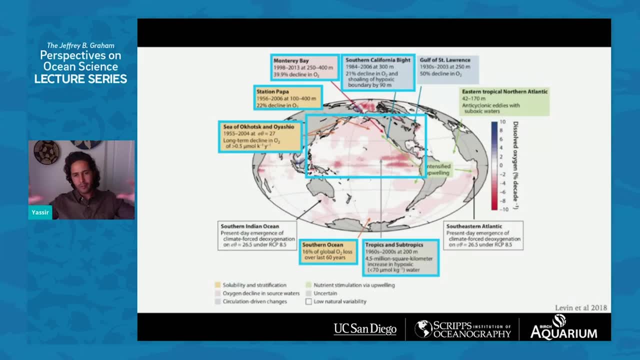 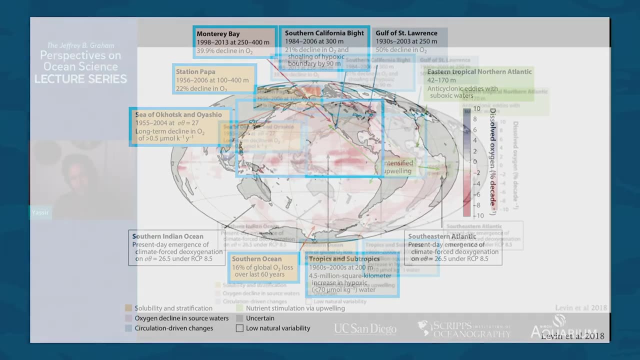 one of the longest time series recording oxygen. there's been a 20% decline in oxygen. So there's some pretty large changes regionally that are superimposed on sort of a smaller decline globally. But there's also a lot of uncertainties in some of these numbers. For example in the tropics, the observations can 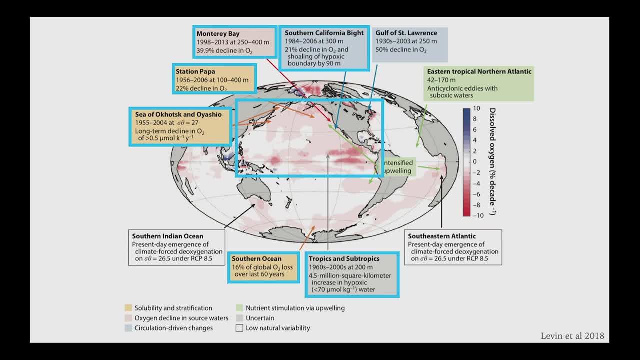 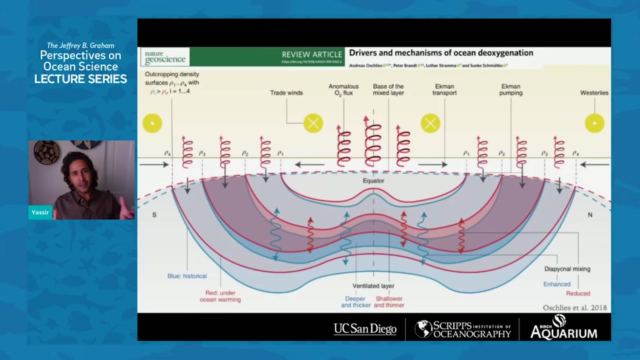 be sparse, And so there's still a lot of work going into figuring out how robust are some of these trends and how much more observation we can get out of new methods. The main mechanism by which oxygen is being lost because of warming one. we said earlier that a warmer ocean can hold. 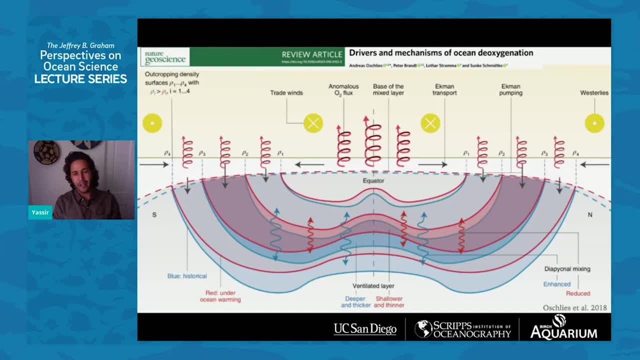 less gas and that's the gas solubility components of the equation. That's just thermodynamics, but that only accounts for about 15 to about 50% of the change. A lot of the change is going to happen because of the circulation effects and the biology effect. 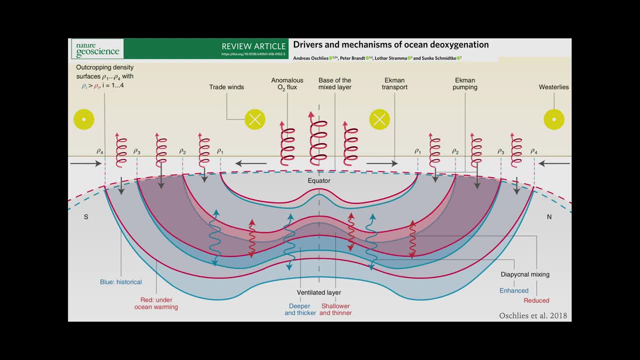 And this is an illustration, and it looks pretty complex with all kinds of arrows, but essentially, if you follow these arrows, these, for example, here are the mid latitudes, the high latitude or the wide attitude, and this is a state of the movement map. What you can see here is that, by clay movement based on SOP. 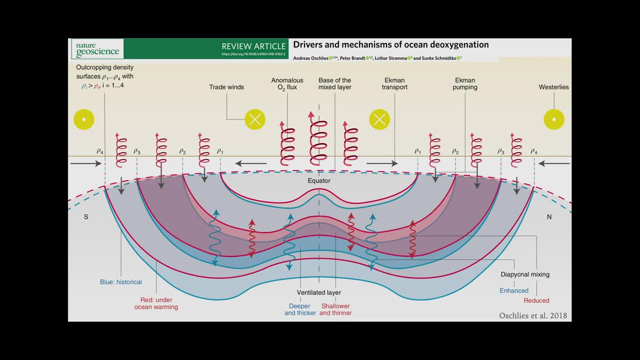 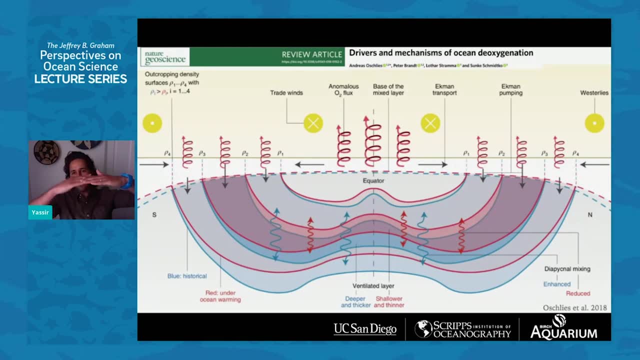 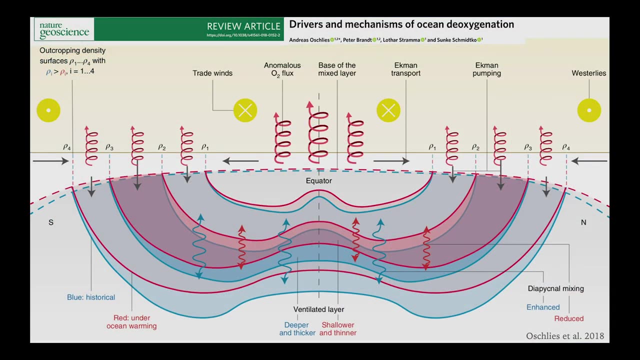 where water goes into the ocean's interior, And so, as the ocean warms, the upper ocean becomes more stratified, becomes harder to mix waters between these different isopignols or different layers of same density, And the upper ocean becomes more stratified. 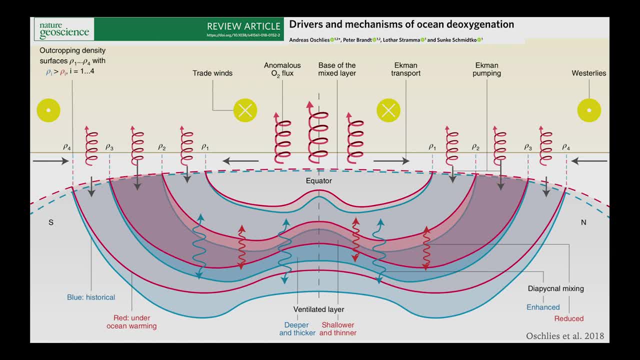 there's less ventilation to the ocean's interior. So that kind of creates even more time for these microbes to respire oxygen and less oxygen supply to the ocean's interior. So that's one mechanism by which we think that the oxygen immune zones are gonna be expanding. 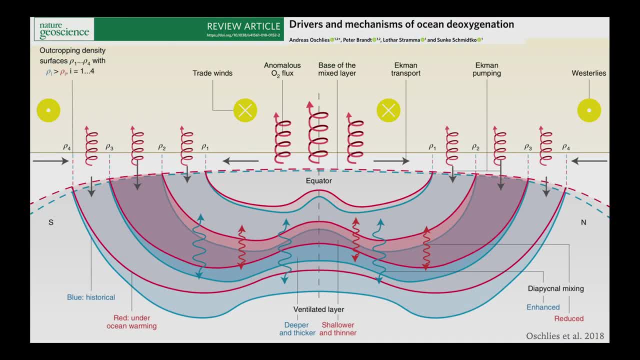 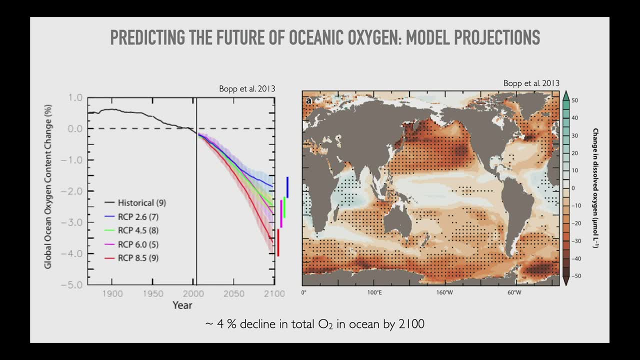 as the ocean warms, We can turn to models like climate models to sort of get a general understanding of how the Earth system gonna respond to this warming To the right is a combination of different models that were submitted to the IPCC report. The IPCC report is an intergovernmental 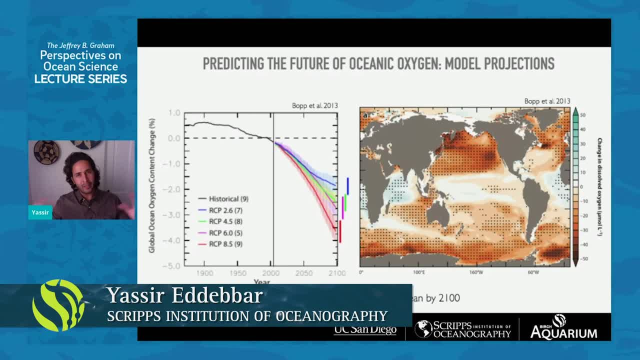 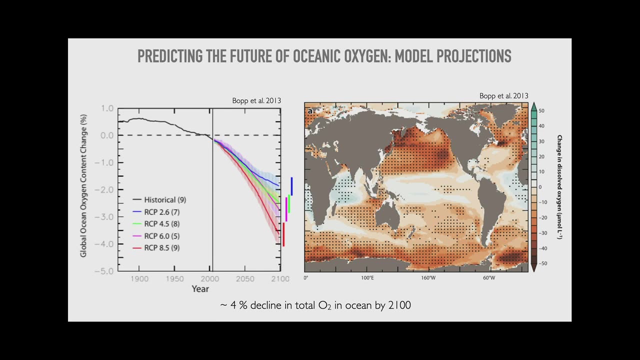 panel of expert that provide input from the literature on latest science And they use Earth system models to try to infer what's gonna happen by the end of 2100.. And what these models are showing us is that, as the ocean warms, there is gonna be less oxygen in the layer. 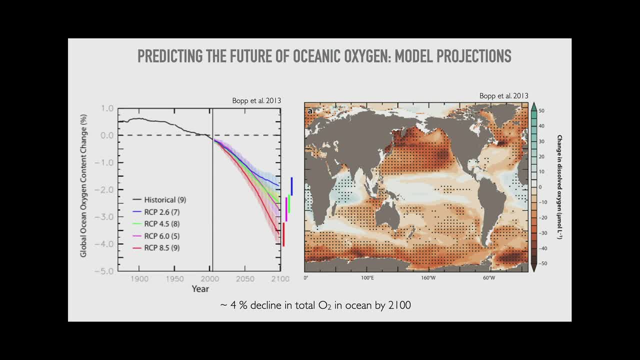 that we call the thermoclines. This is the depth of about 200 to 600 meter depth. This is typically where you can find a lot of these oxygen immune zones. They show that there's less and less oxygen in the high latitudes. 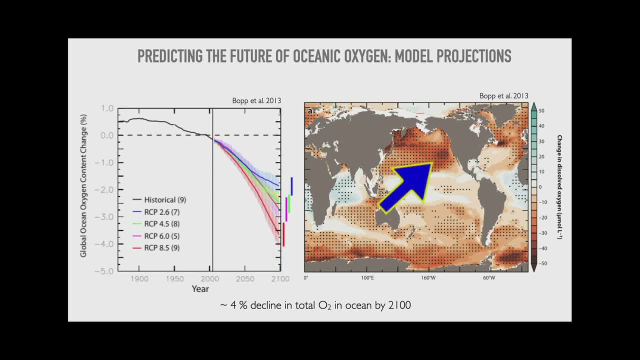 For example, here in the Southern Ocean, in the North Pacific and in the mid latitudes and the North Atlantic, And that's the rate of the oxygen decline here shown for the global oxygen content change in percentage. So by 2100, depending on what scenario you pick. 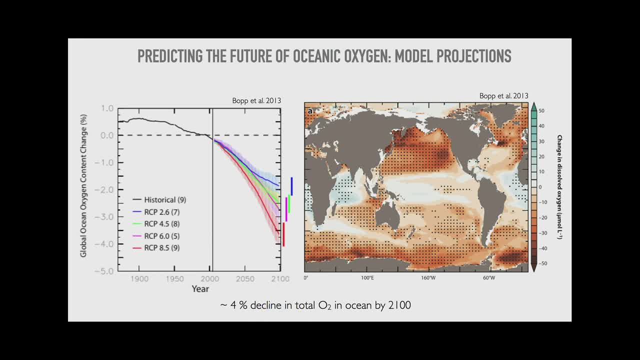 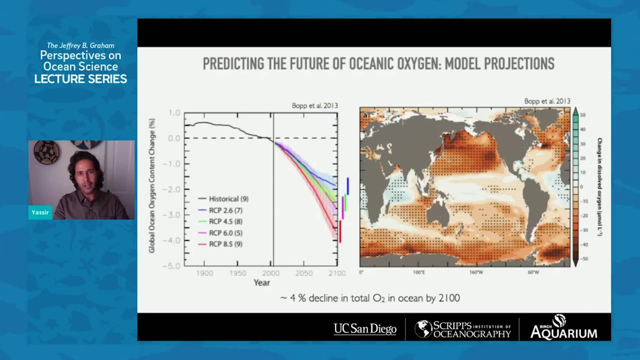 if it's low emission scenario in blue- or a high emission scenario, which is business as usual. we're looking at anywhere from an additional 2% to 4% change in the oceanic oxygen inventory, So the amount of oxygen that might be lost in the future. 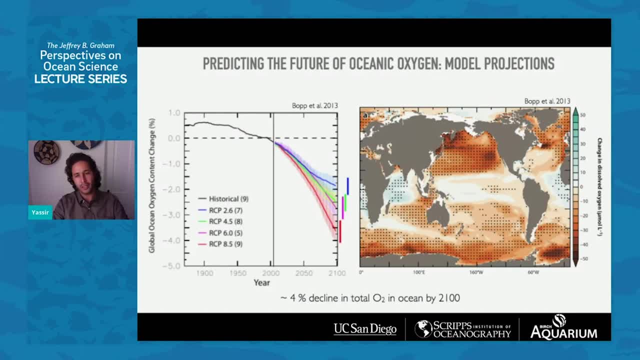 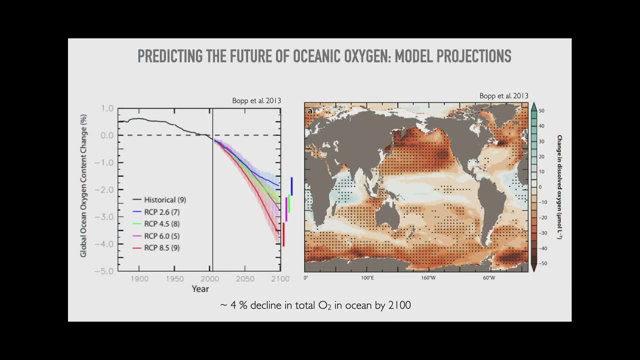 depends on how much greenhouse gas emission we can make in the future. Well, one interesting thing that I wanna point your eyes to is this region in the low latitudes. So we'll talk about that in a bit. but the models don't really agree very much. 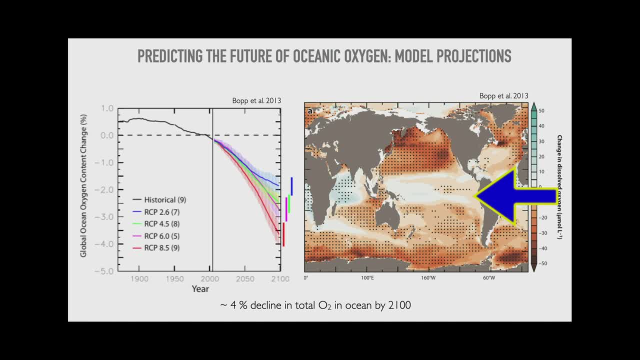 on what's gonna happen in the low latitudes. The agreement between the models is shown here in dots. So where there's a lot of agreement between the models, you'll see dots and you'll also see a decrease in oxygen, Whereas in the low latitudes, 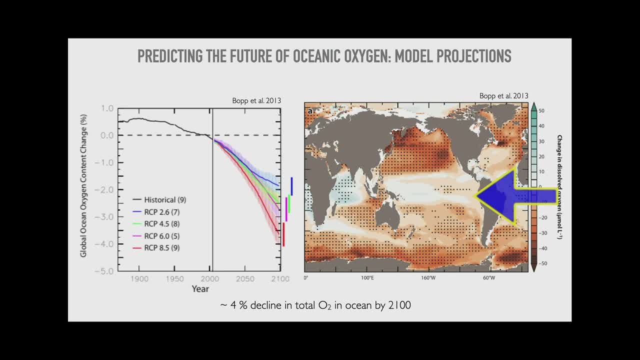 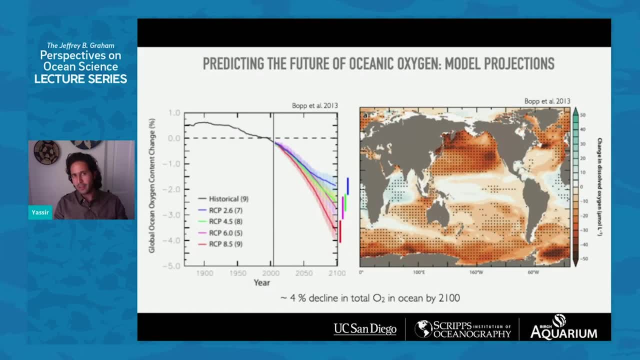 there is generally low disagreement between the models, and some of them even show that there's gonna be an increase in oxygen in these oxygen minimum zones. So the picture that the models are giving us is really complex. but models are just models, And so we have to use. 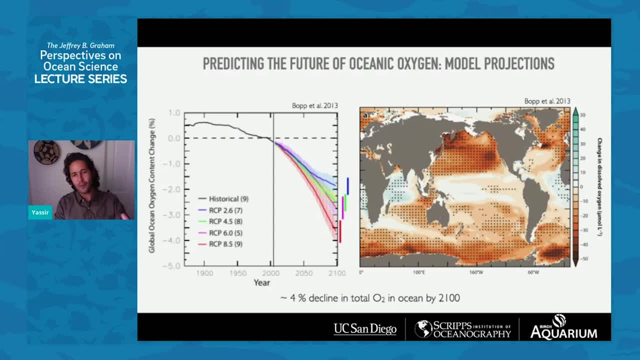 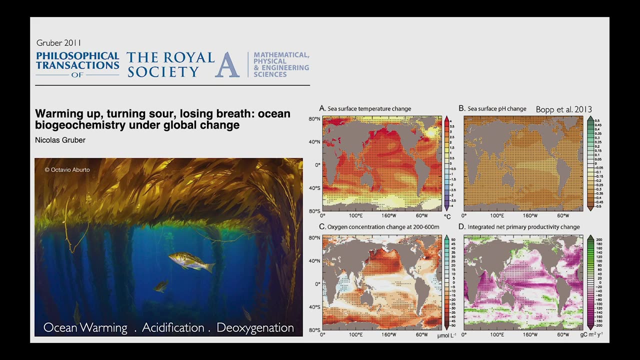 use them with a certain amount of caution. We also have to root our understanding of the earth system in observation first, but get some information from the models. Then I just wanna sort of point out that the oxygen changes that I've shown in these models 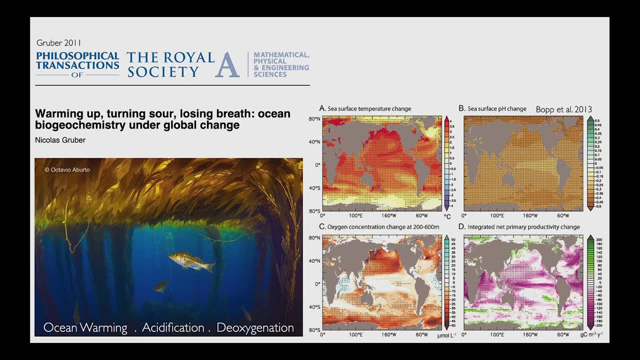 are just one of many other impacts that we expect from a warming planet. We know that the earth system is gonna warm up and the sea surface temperature and the oceans interior are gonna warm, So there's a lot of agreement between models on that warming. 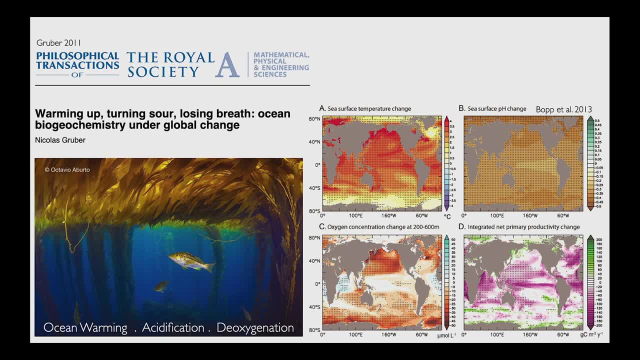 We also know that the additional CO2 in the atmosphere is gonna cause more acidification or a decrease in pH, And that's also pretty well understood. A lot of it is driven by carbonate chemistry. That's really well understood. And then, finally, we also think that there's gonna be changes. 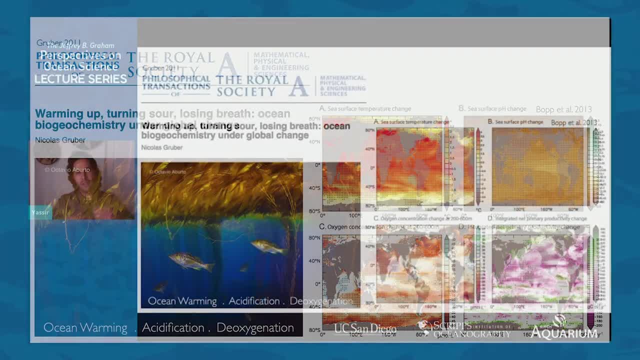 in primary productivity. So the amount of nutrients that come onto the surface and the amount of productivity from phytoplankton bloom and the amount of nitrogen that comes out of the surface. So the amount of nutrients that come out to the surface and the amount of productivity from phytoplankton bloom. 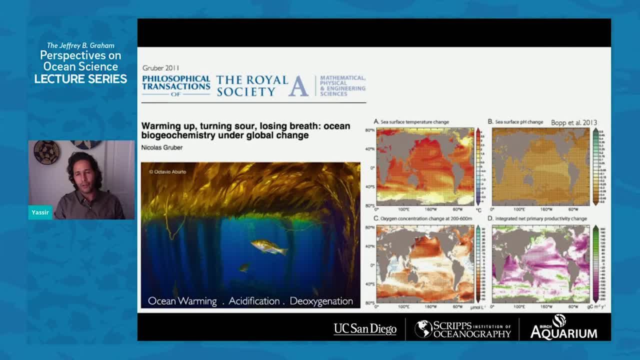 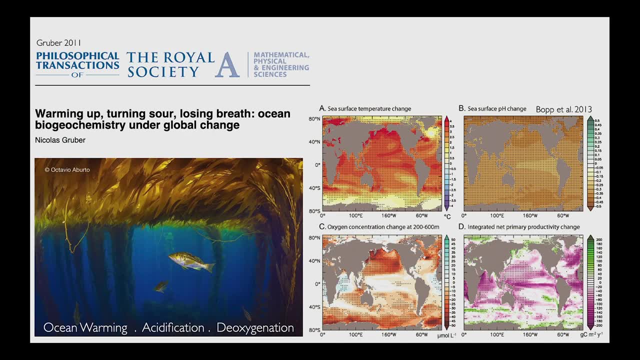 might change And that's kind of depends on circulation and warming and variety of different processes. But that's even less certain than what's happening with oxygen. But I just wanna sort of show that there's way more than just one impact And oxygen is just one of them. 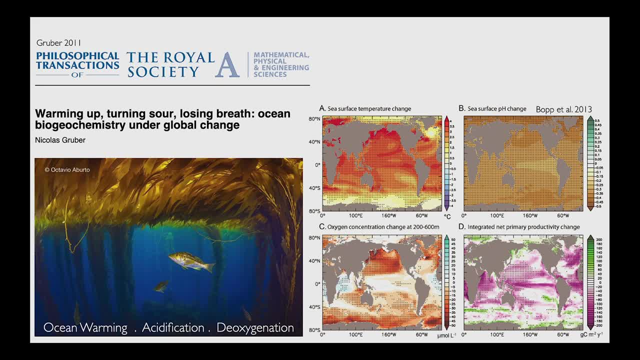 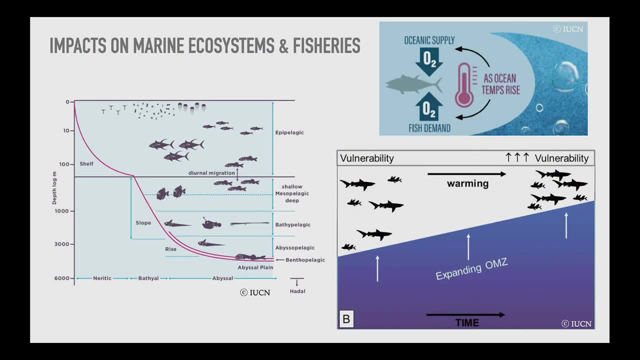 but it's also one of the most important ones And we have to study it sort of in concert with these other impacts And as a scientist, I'm really sure that I'm gonna be able to do some really fascinating this topic from a scientific standpoint. 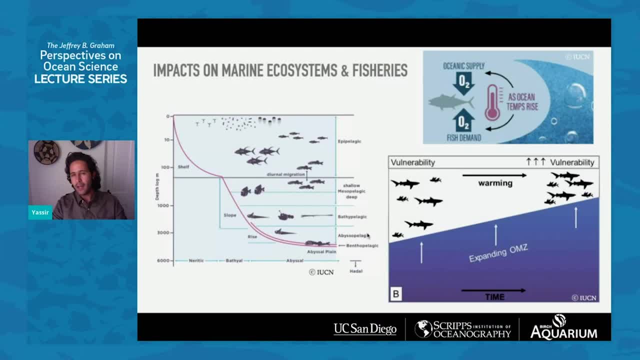 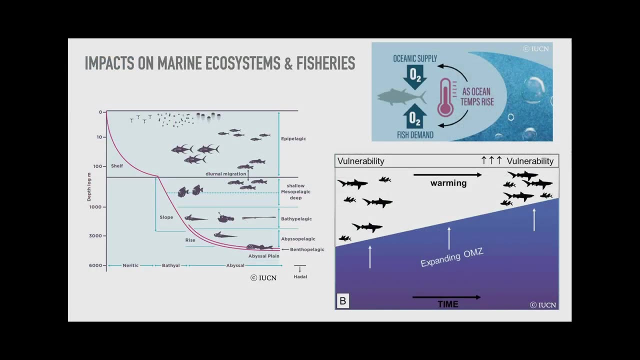 but I'm also concerned about this impact in marine ecosystems. Marine ecosystems are really complex, and especially the interaction between different communities, vertically and also laterally. And so, as the ocean warms, not only is the oxygen supply or the oxygen in the oceans. 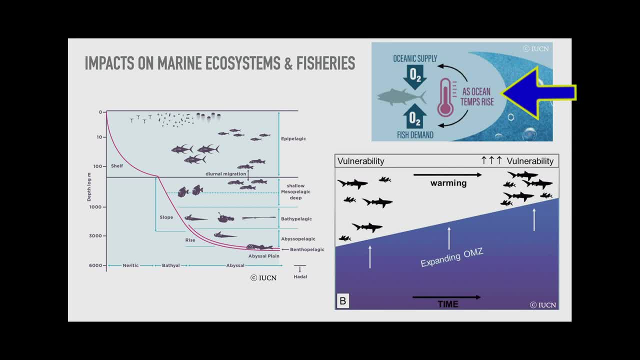 how water is gonna decrease. the oxygen demand from fish is also gonna increase because it's warmer And as these OMZs are expanding, these marine ecosystems are gonna get squashed further up. So the hypoxic depths as it shows. 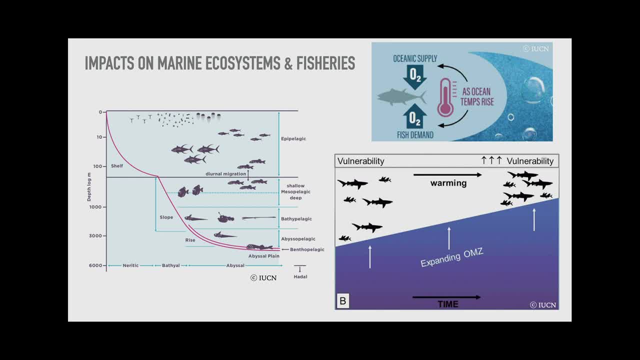 is gonna create less space for these different marine ecosystems to coexist, So that means that preys are gonna become more vulnerable to predators. Fish as a general is gonna be more vulnerable to fisheries. A lot of this is a lot of it's work in progress. 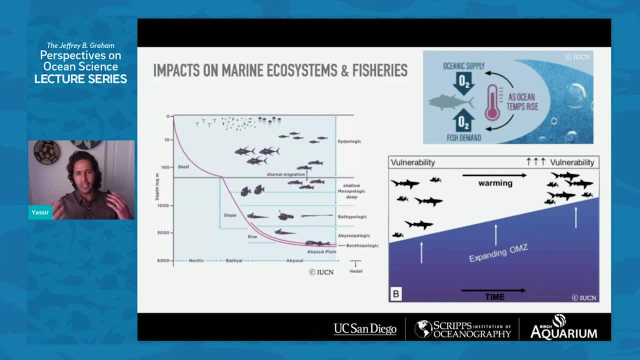 And we're really just starting to understand the impacts of changes in oxygen on not only ecosystem dynamics but also marine organism health, including vision, And we're gonna hopefully hear soon within this lecture series on some of the biological impacts of these oxygen and OMZLN expansion. 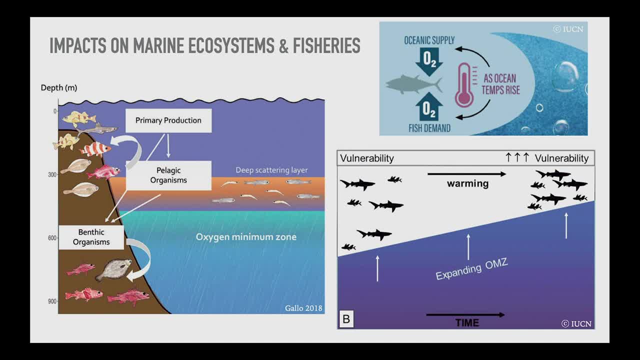 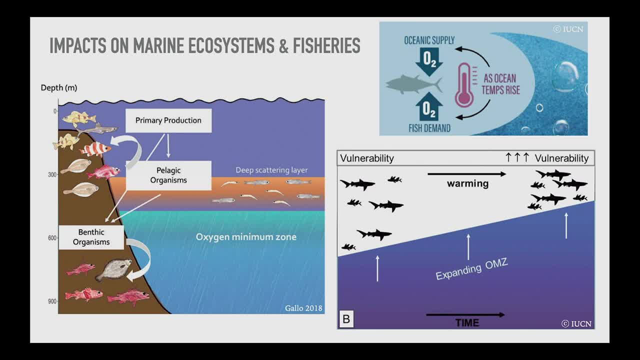 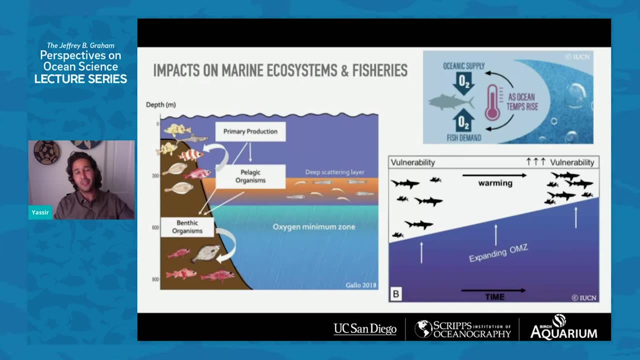 or changes in decoupling between pelagic organisms, those that live offshore versus those that live on the bathhouse on the ocean's floor. So there's a lot of exciting work that's happening, that's trying to understand how marine ecosystems are going to adapt or react to these changes in the ocean's environment. 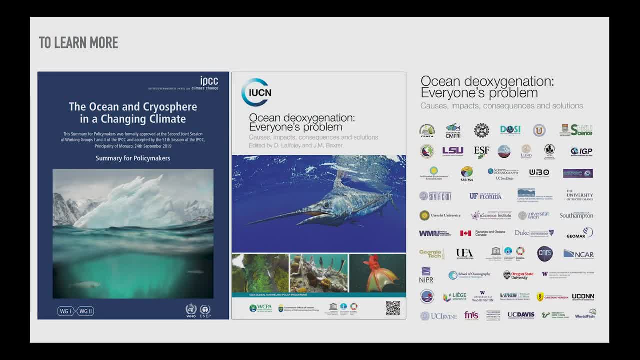 If you want to learn more, there's some great resources. One is the most recent ocean cryosphere report that's been done by the IPCC And there they've assembled a lot of the most recent literature on what's happening in our oceans, including oxygen. 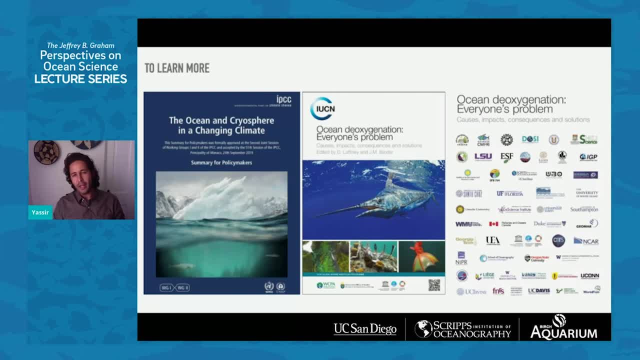 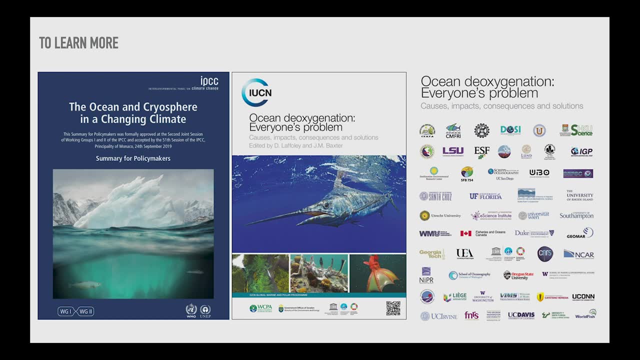 It's got a very. It's a thorough section on oxygen And, if you want to get into even more detail, the International Union for the Conservation of Nature has published a report recently and scripts scientists and scientists from around the world have contributed to sort of summarizing a lot of these scientific problems. 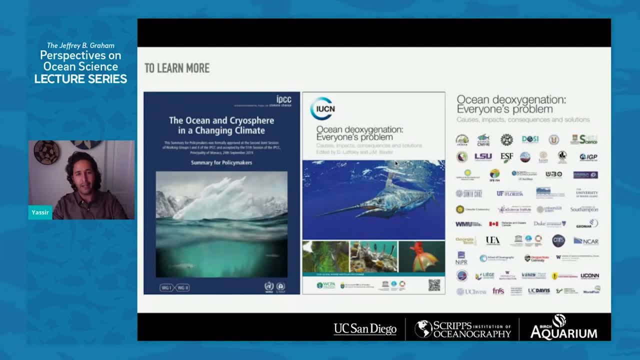 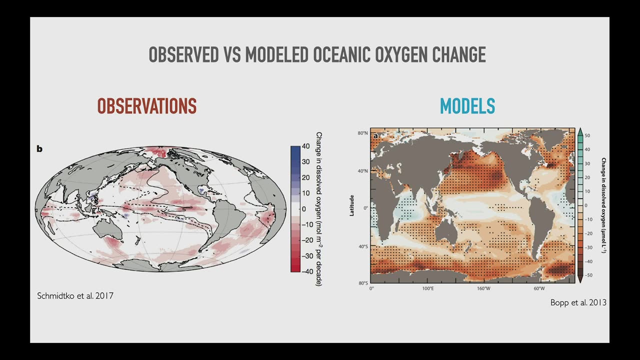 in this report And I strongly recommend to look it up online and get caught up with the science behind it. There's a lot of interesting publications for marine ecosystems that we expect from this problem, And oxygen is really tough because it includes a bunch of different processes happening at. 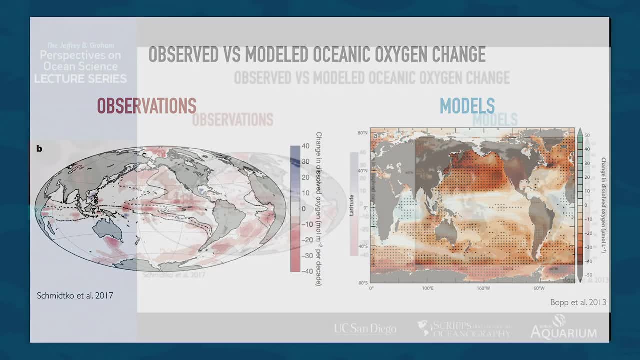 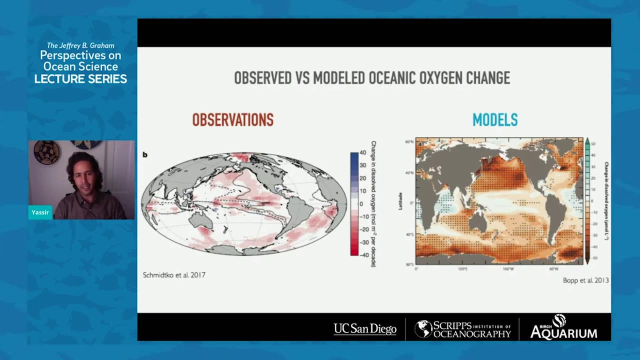 once So: ocean circulation, chemistry, biology- And it's also a problem that we don't fully understand yet. The science behind it is still somewhat young, And you can see that, for example, in this discrepancy between what the observations are showing and what the models are showing. 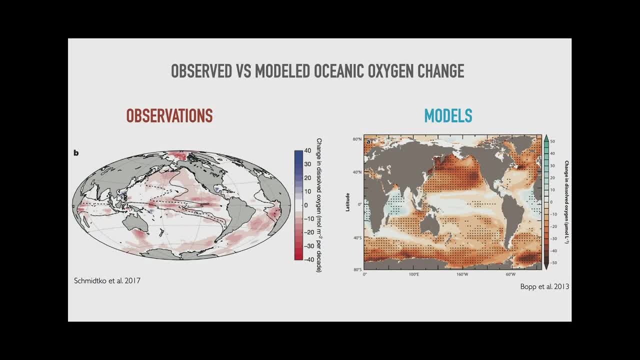 And you can see that, for example, in this discrepancy between what the observations are showing and what the models are showing. I've sort of referred to earlier that the observations are showing a substantial amount of oxygen loss in the tropics, Whereas the models mostly show very little changes and even a positive increase in oxygen. 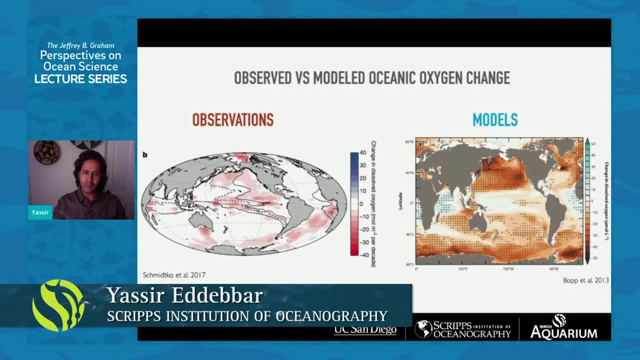 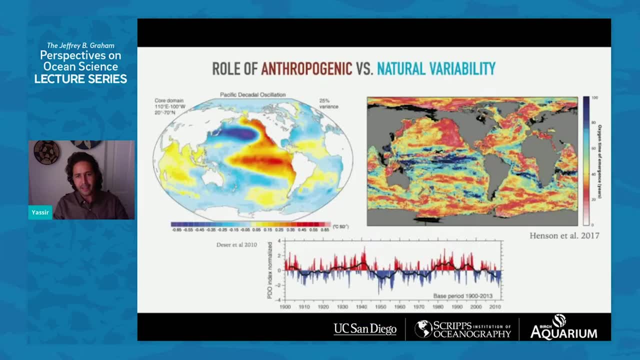 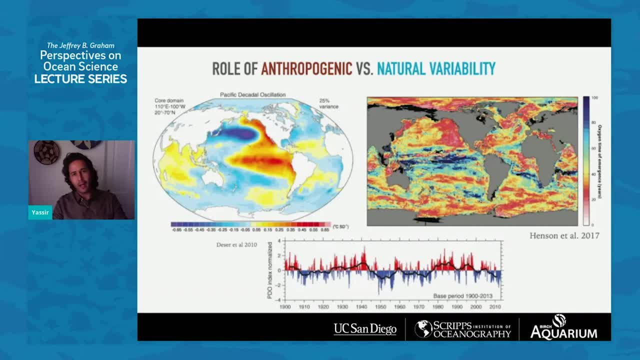 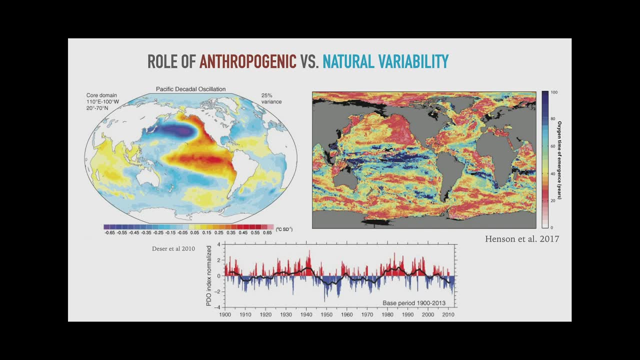 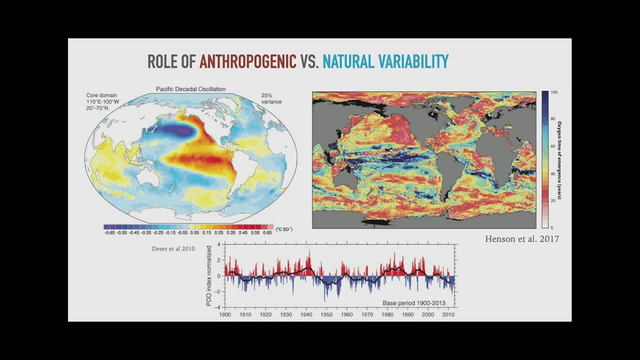 role of natural variability. For example, here to the left I'm showing sea surface temperatures that are associated with natural variability phenomena. we call Pacific Decadal Oscillations, And it's just an index that we use to describe decades that are typically cold. 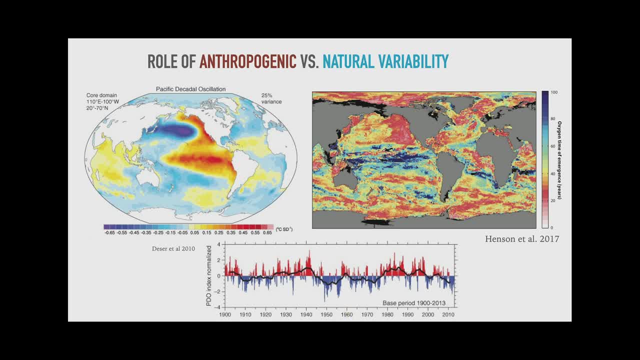 For example, the 1960s to 1970s, and decades that are warm, for example the 1970s through the 1990s, And these natural modes of variability, like the Pacific Decadal Oscillation, El Nino, that many of you are familiar with. 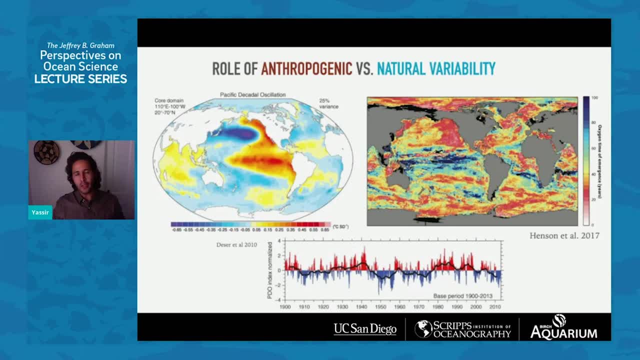 they induce a lot of variability, not only in temperature, but also in the biology and the chemistry of the ocean. So what that does is it really creates a problem in trying to identify what is human-driven, what is the change in the oxygen that's driven by human warming, and what's natural. 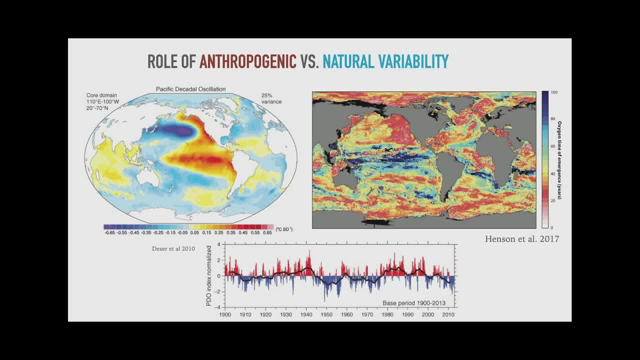 And that's something that really fascinates me and many of my colleagues. but it also makes it really hard to detect the anthropogenic signals in the ocean And to the right here I'm showing what we call the time of emergence, which is really the time by which the anthropogenic signal 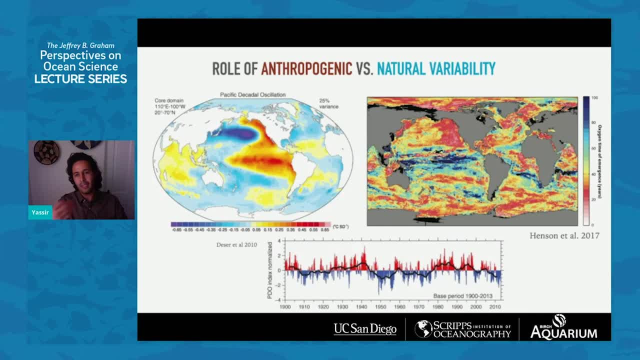 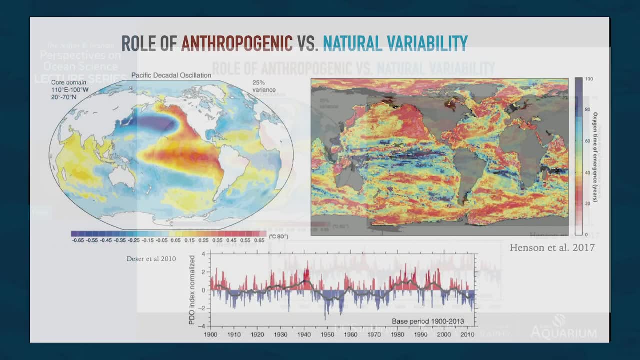 or the anthropogenic impacts on oxygen are going to be detected in measurements, And sometimes we might not be able to find that for another 50 or 100 years, for example over regions in the tropical Pacific, But in other places, like in the northern tropical Pacific. 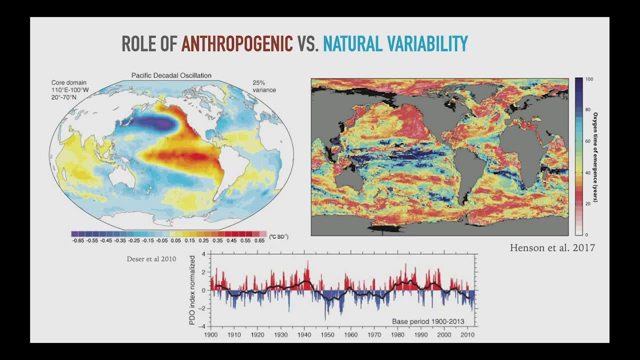 in the Atlantic or Southern Ocean. this paper here shows that we can expect to see the influence of human warming on oxygen in the next 10 years, or even now, or even the next 20 or 30 years. So natural variability is really important. 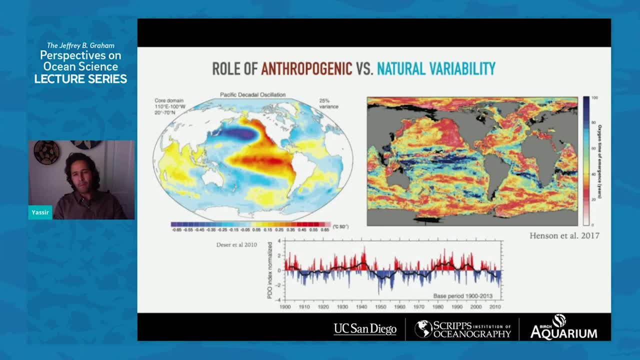 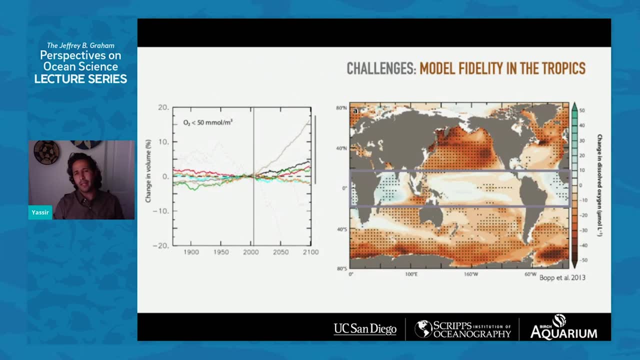 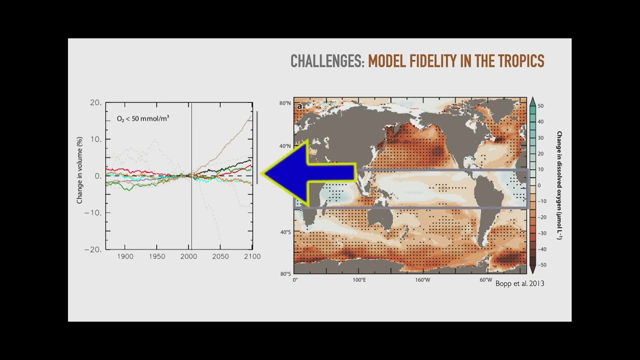 It's one of the biggest changes. It's one of the biggest challenges that we face. Another problem is that the models themselves don't do so well in the tropics, When you look at their projections here for regions that are hypoxic below, say, 50 millimole per meter cube. 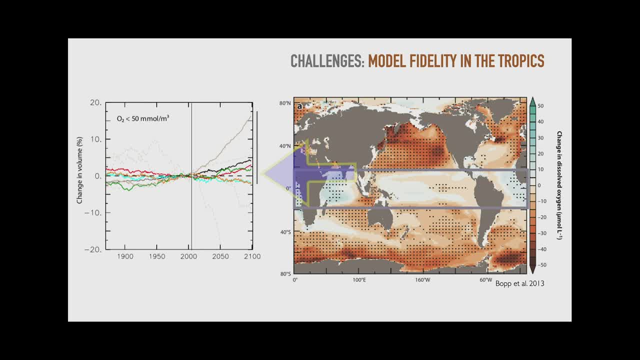 the behavior of different models and different colors here show different trajectory for a different model. Some models show that the volume of the hypoxic or the oxygen zone is going to increase- in certain models sometimes really increase, And for other models it shows very little change. 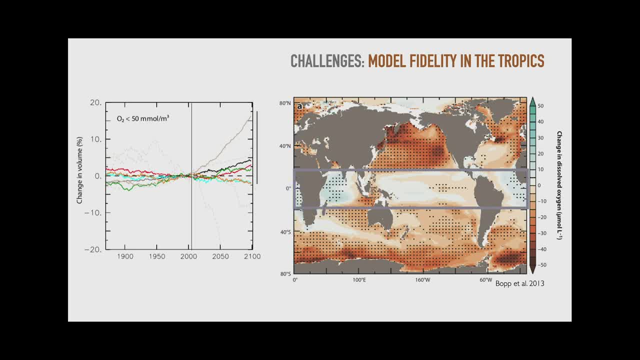 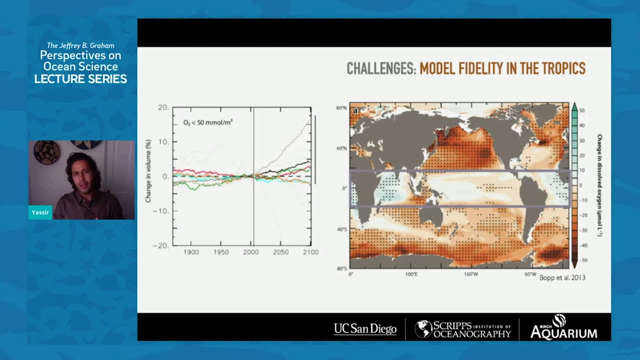 if not a decrease in the volume of the oxygen zone or an increase in the oxygen content in that region. So each model is going to show a different future in that region, in part because of their biases And the model biases here. what I mean by bias is that they're not reproducing the mean state. 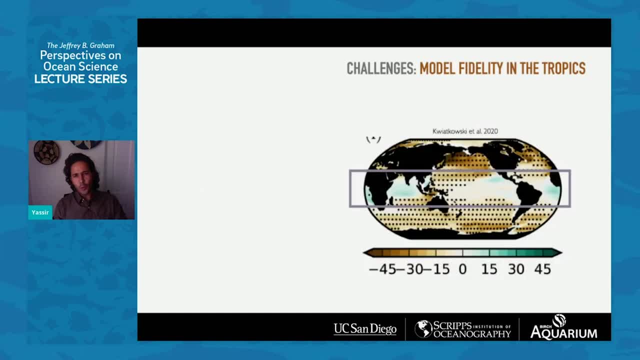 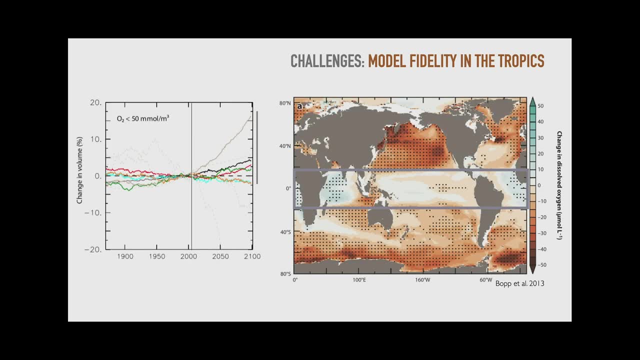 or the processes in that region really well. So how does that change, for example, from one generation of model to the next? What I've shown here is models from the last IPCC report, And so there's been a lot of work over the last seven to ten years. 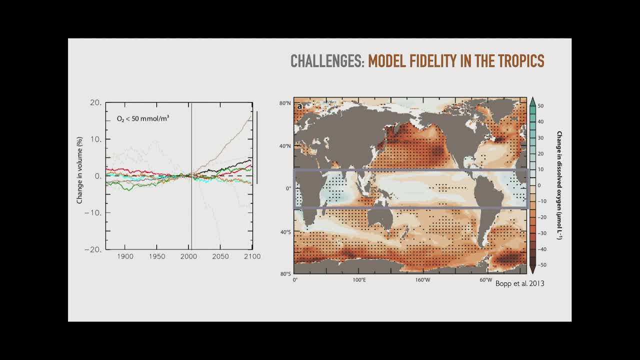 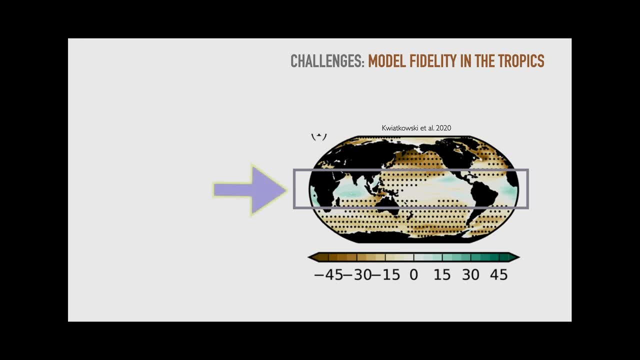 to try to improve how these models represent ocean circulation processes, But the most recent paper- this just came out last week- shows that models are still doing pretty poorly in that region And they're also still disagreeing on what's going to happen in the tropical Pacific. 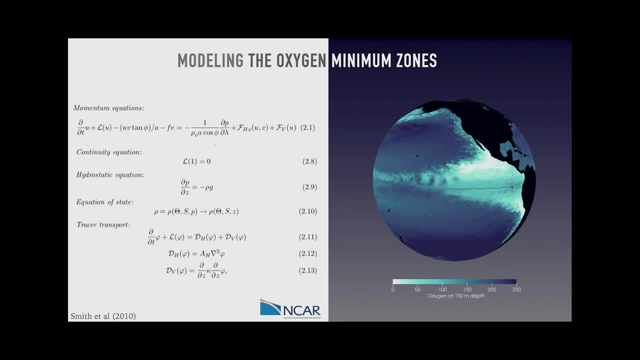 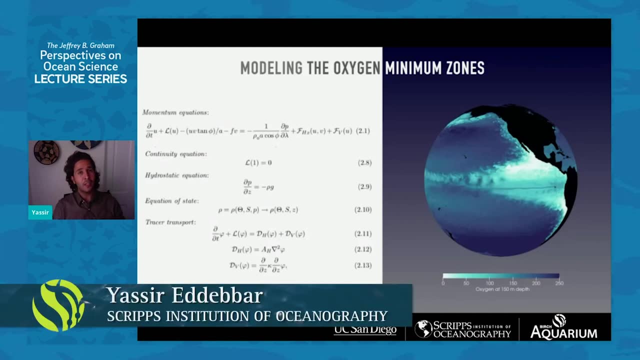 So a big challenge is try to understand what's happening in tropical Pacific. How can we better model the oxygen zones in that region? And one big challenge there has been computational resources In order to represent the oxygen zones. we have to get really small scale circulation features right. 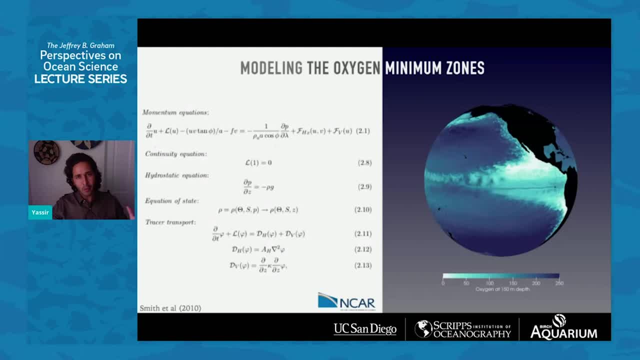 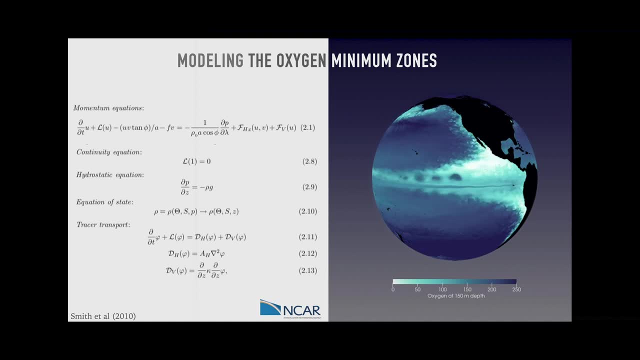 For example, eddies or equatorial currents like the equatorial, and we have a really good understanding of global ocean circulation in these climate models. But at regional scales we're now really starting to understand how these smaller scale features are impacting the oxygen distribution. 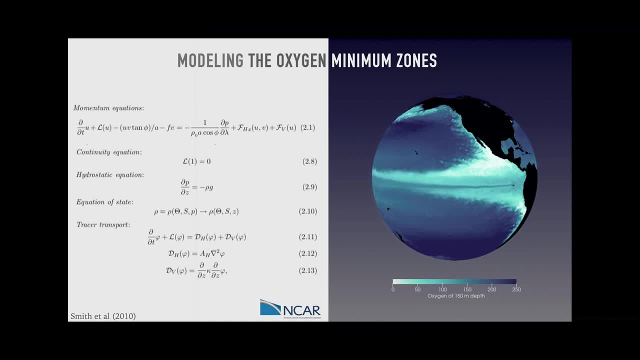 You can see these beautiful patterns starting to emerge here along the coast of North America. Equatorial undercurrents bring in oxygen to the Eastern Pacific eddies, changing the extent of the oxygen zone. So it's really an interesting time to be a scientist. 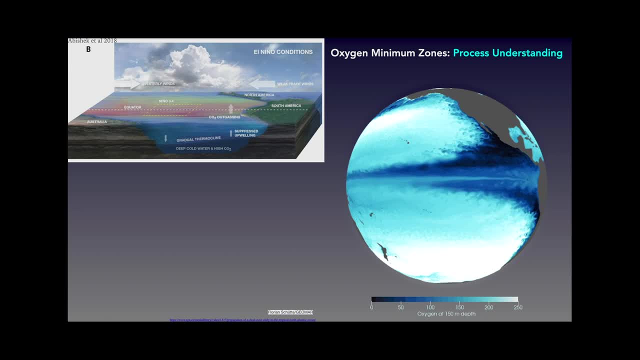 Another really important advantage of using models that allow us better process understanding of natural variability. We can run a model without any anthropogenic forcing and just try to understand how El Niño is going to impact the oxygen minimum zone, how the Pacific Decadal Oscillation might impact an oxygen minimum zone. 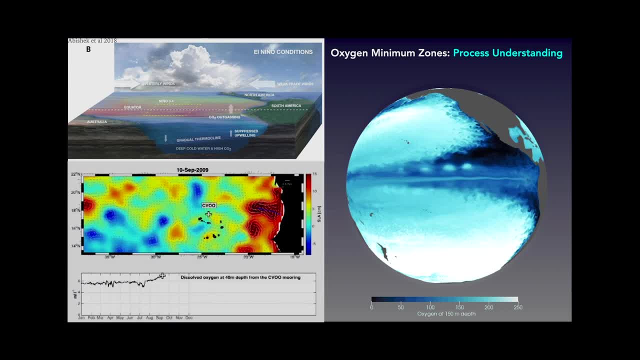 or even how these small eddies, for example this observed eddy, which is like a storm that happens in the ocean that traps low oxygen water and transports it, and it's been observed here in the Cape Verde Ocean Observatory to lead to very low oxygen values for almost a month in that region. 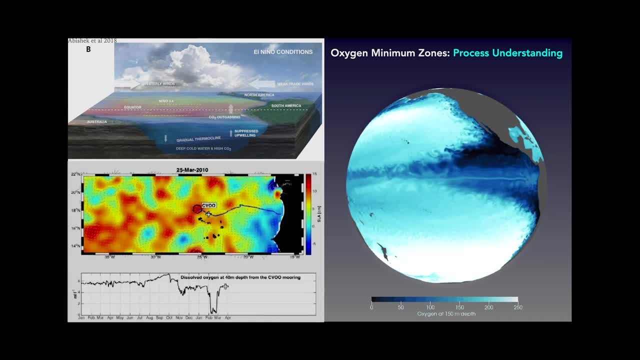 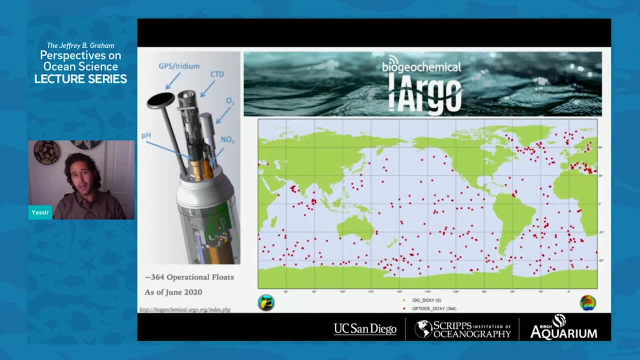 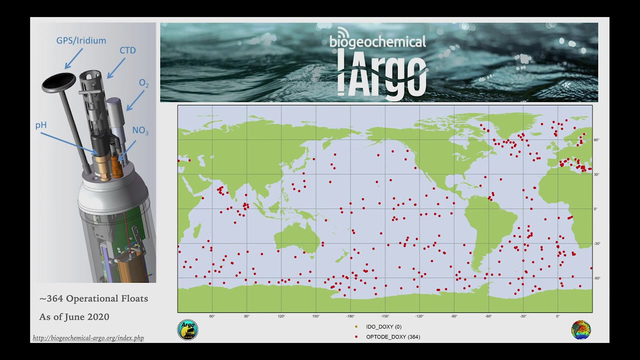 So models are really critical in trying to help us understand what's happening and sort of get a better idea of the natural versus the anthropogenic component. Now, finally, the observations have been sparse for the last five or six decades, but there's an exciting new program called Biogeochemical Argo Program. 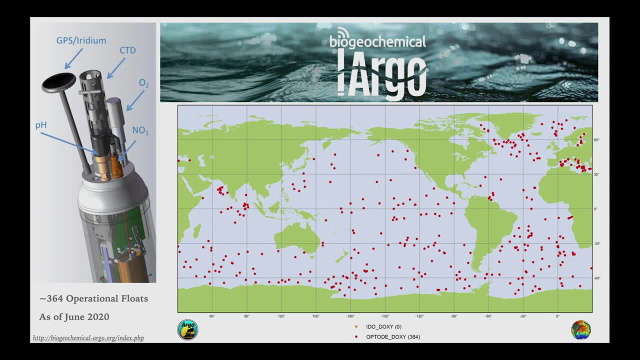 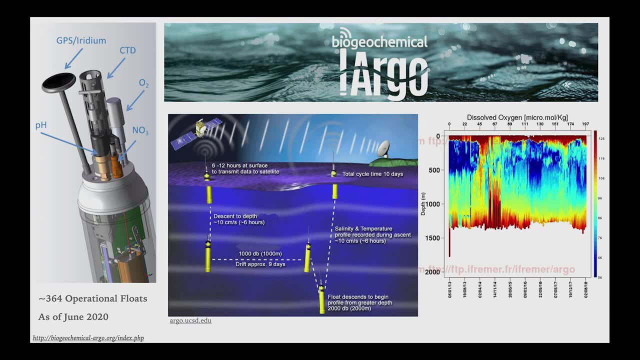 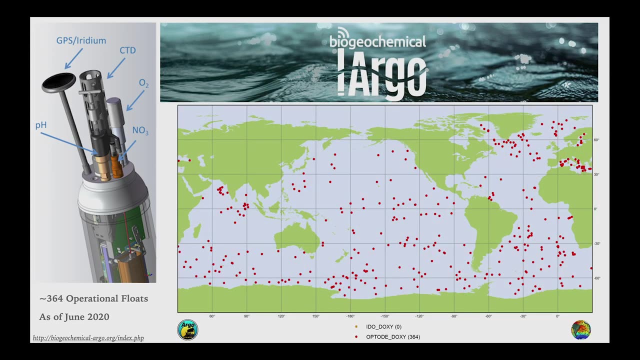 And some of you have heard of this as the Argo Program, where a float goes up and down the ocean's interior and records temperature and salinity and delivers it back to us via satellite. These biogeochemical Argo floats are very similar. 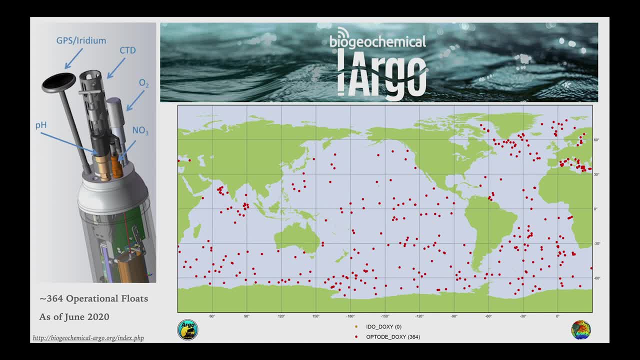 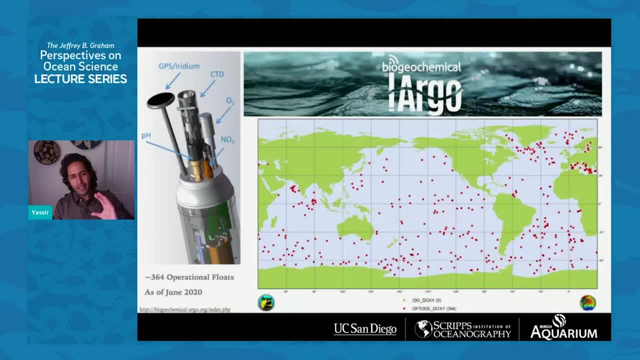 except that they they also record oxygen through a little sensor that you see here to the left And they're going to be really instrumental in trying to record how the oxygen mineral zones are going to evolve in the next 10, 20 years. 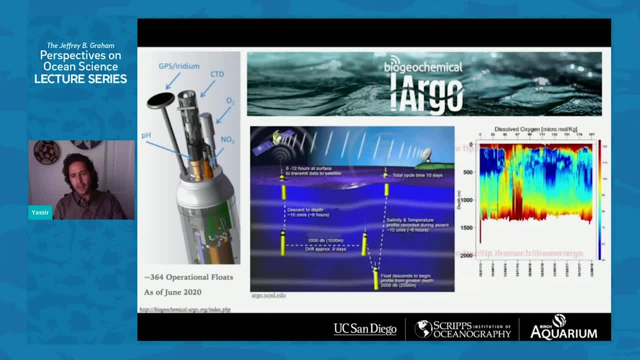 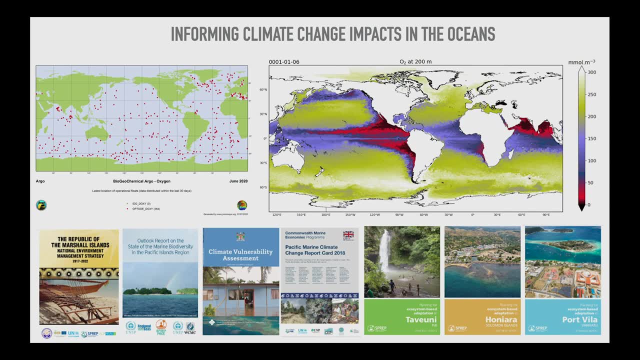 So this is really an exciting new development that me and many colleagues can't wait to get our hands on the data and try to start to work with it. So, to wrap up, I think this is an exciting time to be a scientist. 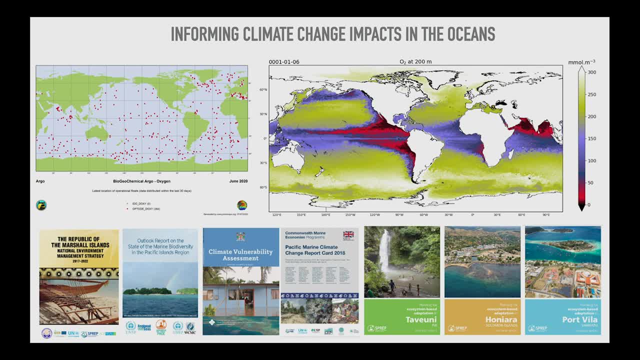 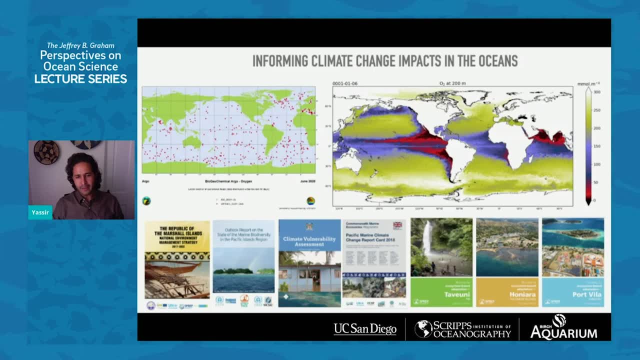 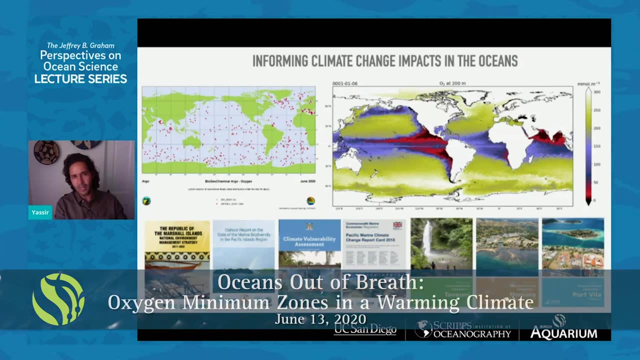 despite all the challenges of few observations in the past or model limitations, there's now more observations than ever. the models are getting better and better And that's kind of really helped us become more prepared to the potential impacts of climate change and also natural climate variability. 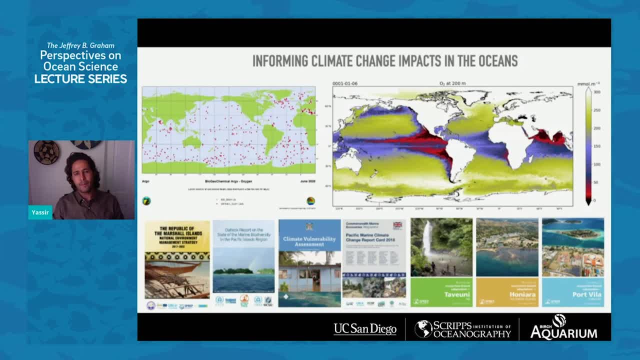 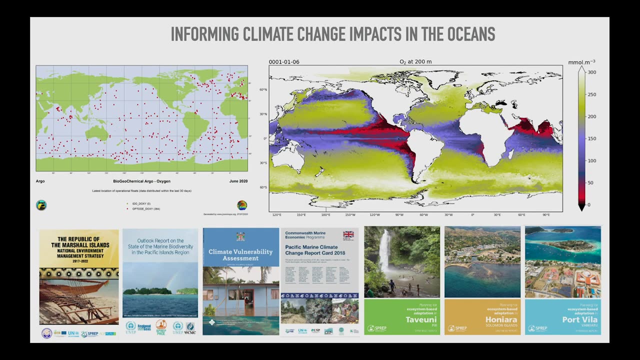 as our community becomes more and more dependent on ocean resources, and especially in small island nations and and nations around the Pacific. As each country begins to develop their own adaptation plan, they're going to need more observations and better models to try to figure out how these resources 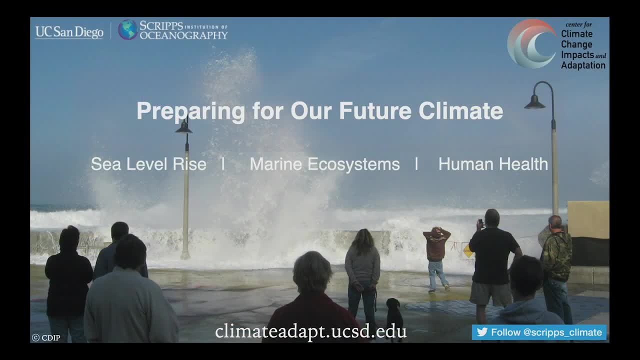 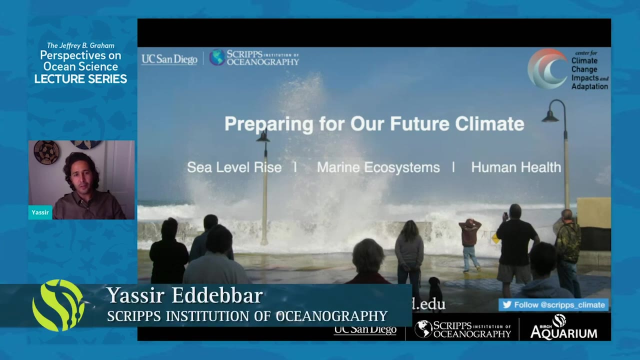 are evolving, And feel free to visit our website at climateadaptucsdedu. This is the website for our Center for Climate Change Impacts and Adaptation, where our focus is try to build preparation through more observations, better models to try to understand how sea level rise is going to evolve in the future. 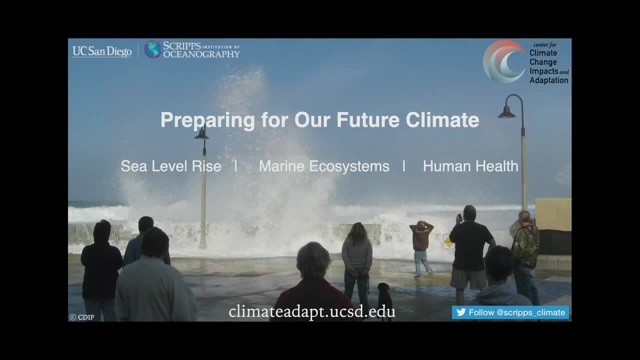 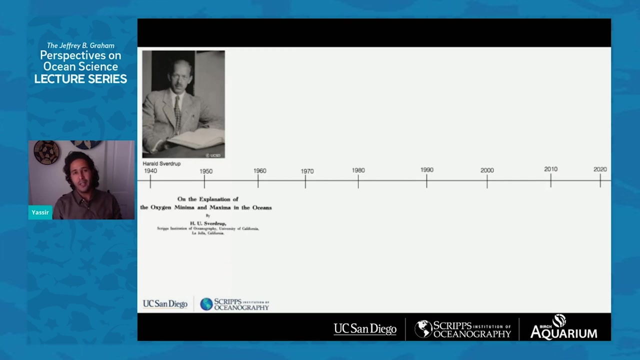 and how it's evolving right now, how these marine ecosystem habitats, especially oxygen, temperature and pH, are evolving, and also human health here on land and in the ocean Sure. I want to sort of reference the long history that Scripps has had in studying oxygen. 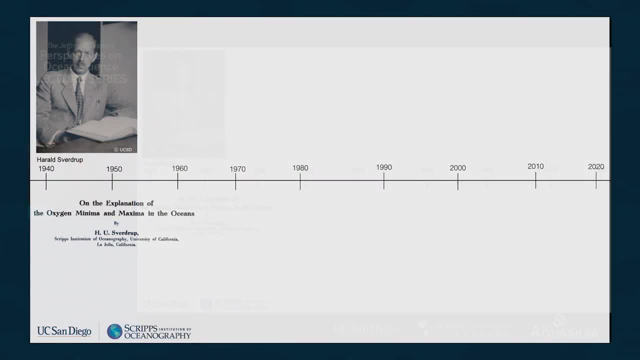 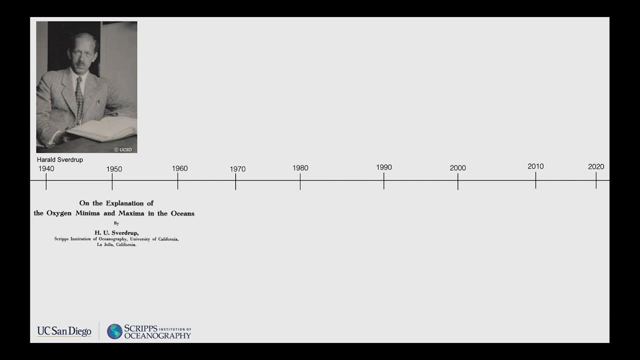 over the last 60 or 70 years. For example, the director of Scripps back in the 1940s, Charles Sparrowdrop, wrote one of the first papers that explained why there's an oxygen minima in the ocean's interior. 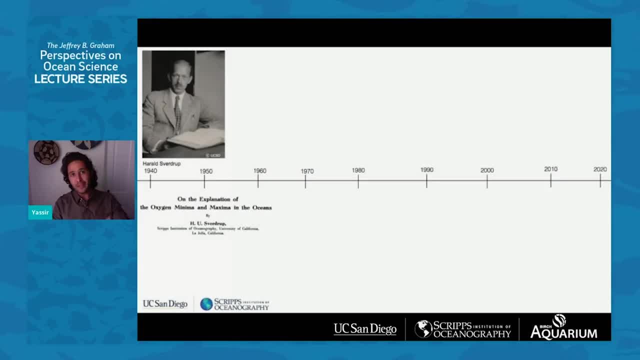 and why there's a maxima, And he was the first to say that biology and chemistry have a major role to play in shaping oxygen in the ocean's interior. There was a major other contribution from a researcher back in the 60s at Scripps. 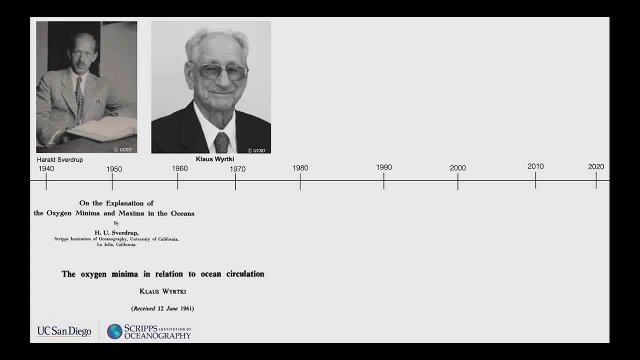 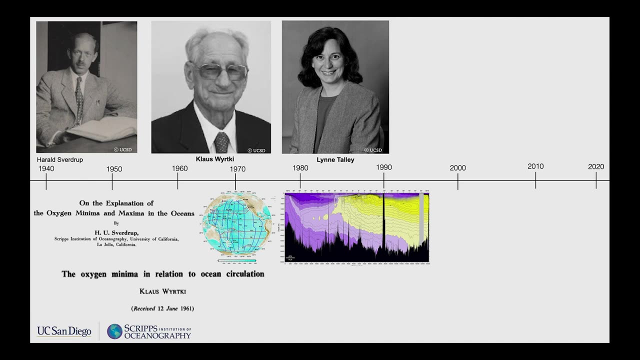 Klaus Wurtke, who highlighted the role of ocean circulation, how this sort of weaker horizontal circulation and more vertical circulation controls the oxygen distribution of the upper ocean. And then really, it wasn't until various cruise sections that detailed the distribution of oxygen in the ocean's interior by people like Professor Lentelli. 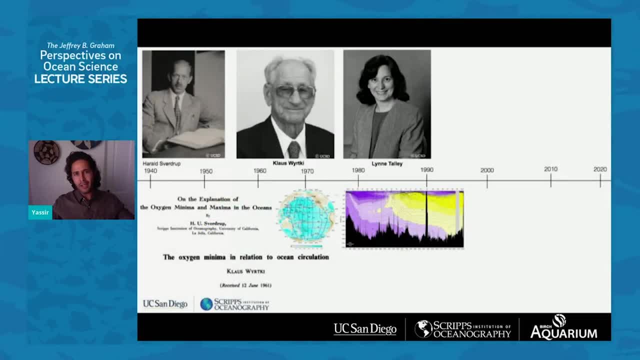 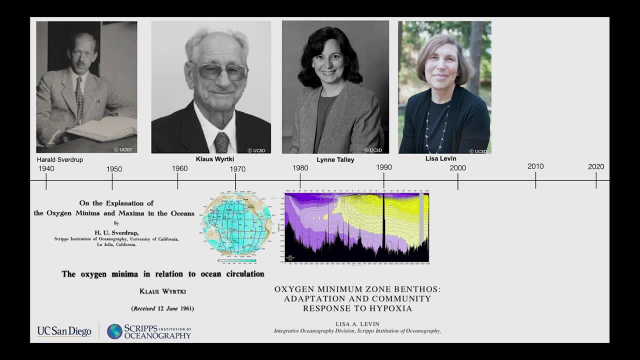 that we've really got a better understanding of just how complex the three-dimensional structure of oxygen is in the ocean, And then, later on, as as more cruises have begun to look at the organisms, looking inside of them. for example, many of the research done by Professor Lisa Levin has looked at the communities that are living within these oxygen. 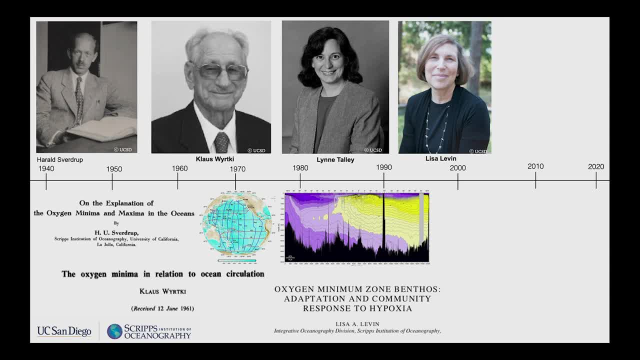 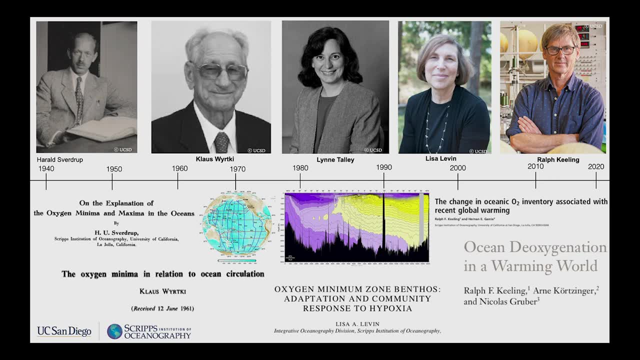 nozzles and how they adapt to such low oxygen values. And then, finally, a major contribution to the field came from Dr Ralph Keeling, who not only measured oxygen in the atmosphere for the first time, but also has done a lot of work in 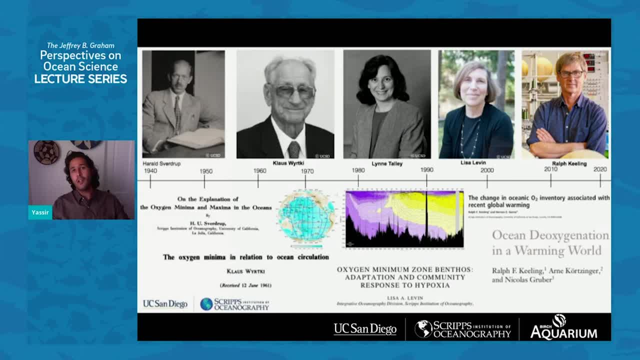 showing how oxygen minimum zones are going to respond to global warming as the anthropogenic CO2 emissions in the atmosphere keep on building up. So I just wanted to give sort of an overview of the incredible role that oceanographers and atmospheric scientists at Scripps have done. 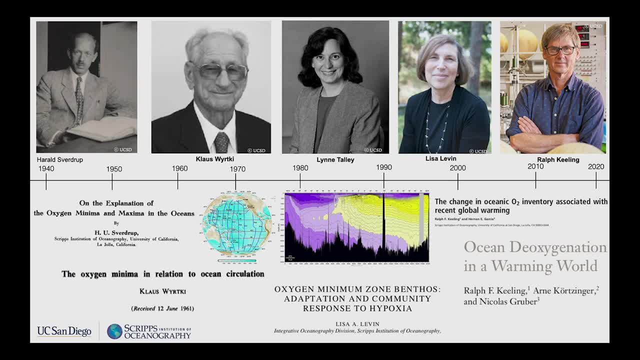 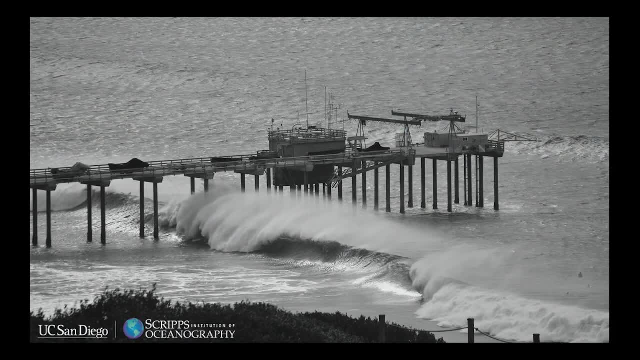 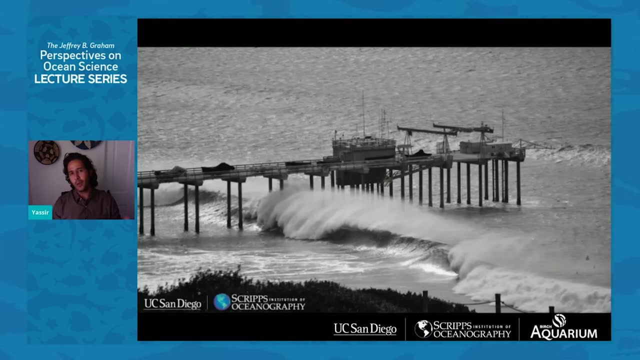 And and I'm really, really honored to also be mentored by many of these people- And the more I learned, the more I realized it's really complex And also it's really important. I've begun to learn that we depend. 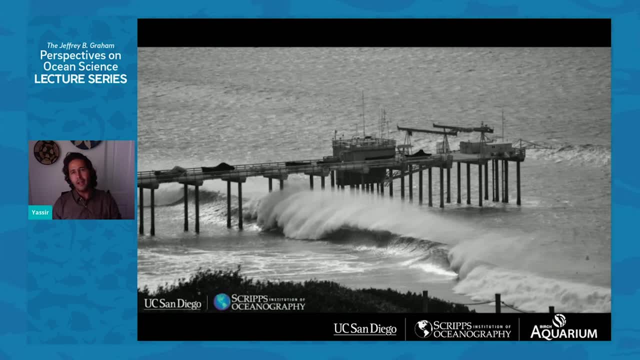 so much on our planet for our well-being. So studying climate and ocean sciences was sort of the perfect way to both be immersed in this element that I really enjoy but also sort of try to understand it so that we better protect it. And, as a surfer, 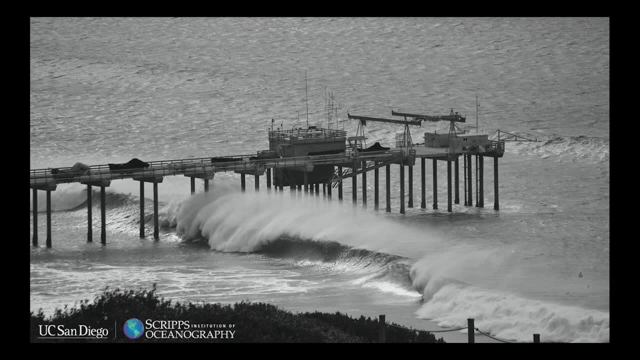 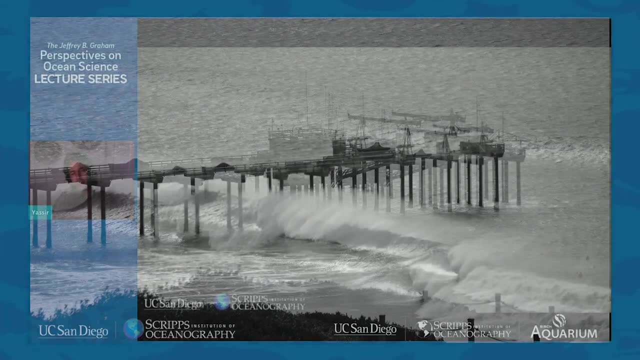 you're out in the ocean, you sort of notice the changes from day to day. You're more aware of pollution events, for example after rain, runoff events. So sort of this combination of curiosity about how the ocean works and the climate system works. 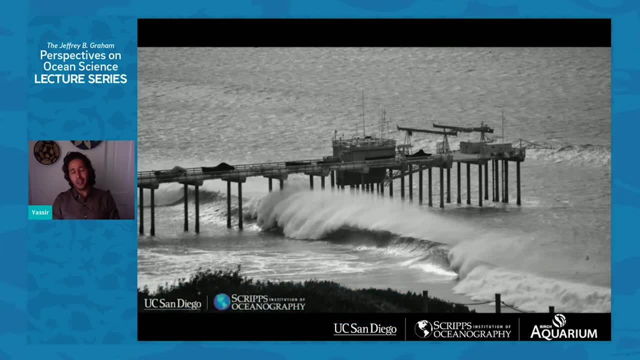 and how different elements- the ocean, the atmosphere- work and also what we can do to protect them with, is pretty unique to climate science and oceanography. So I applied to the best place to do that, and that was Scripps, And I was really lucky to have incredible mentors. 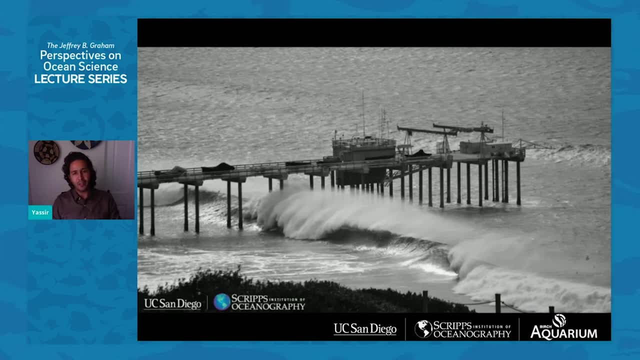 like people I've shown earlier in that timeline- Professor Lisa Levin and Dr Ralph Keeling and many others who sort of helped me develop scientific curiosity, which is really one of the most important drivers of scientific discovery- It's just trying to figure out how things work. 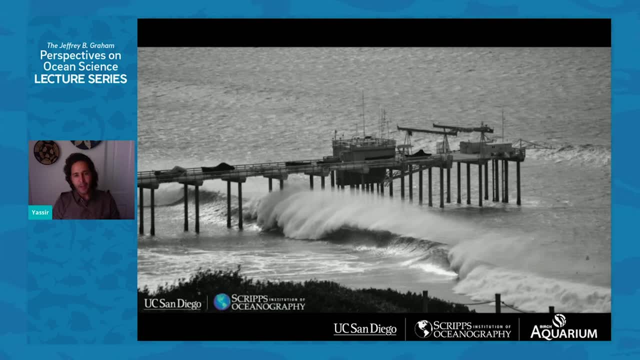 and finding solutions to problems along the way. Oftentimes, when I started my graduate studies, I was on one path and then ended up pursuing very different questions, And while pursuing these different questions, you find different answers than you expect in the first place. 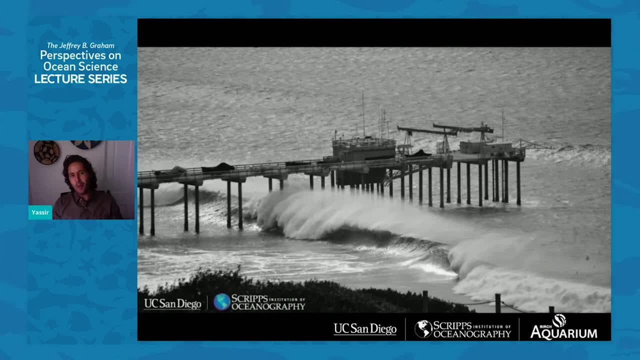 That's been really the common and main thing that I enjoy the most about pursuing ocean sciences in general: just the unexpected. The ocean is full of surprises, full of new discoveries, and we're really just kind of putting our toes in, so to speak. 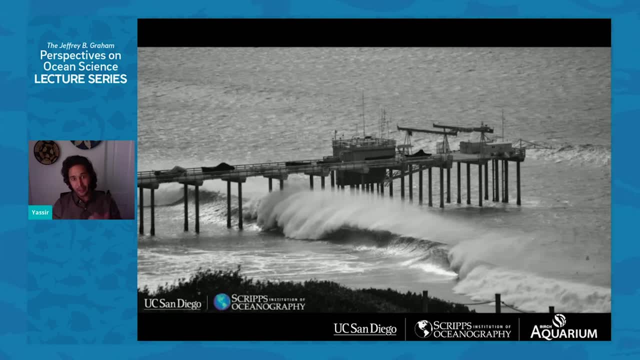 There's a lot more that we can learn and especially a lot more to understand in terms of how it's going to react to our human footprint in terms of pollution or climate change, and also just how it naturally varies and how that impacts us as a society. For example, in cores that we drill from cruises that we take out into the open ocean and we can infer from changes in, for example, marine organism fossils that are stored in those cores at the bottom of the ocean what different species have lived. 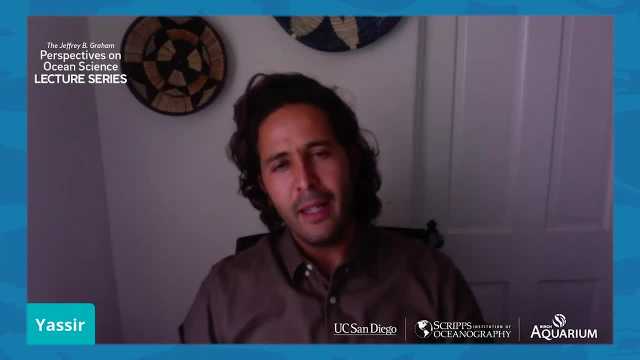 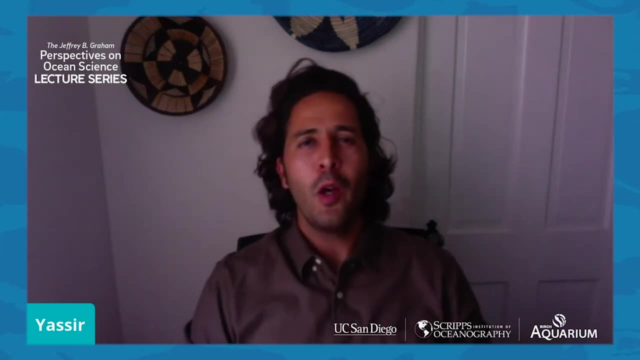 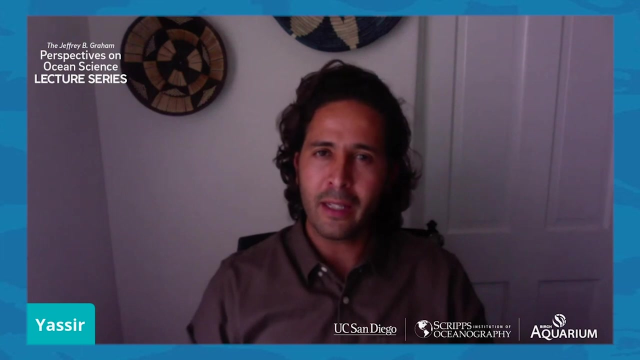 and also how much oxygen was there back then. And one period is the end, the Permian period, some couple hundred million years ago, where oxygen was low and there was a lot of CO2 in the atmosphere from, apparently from enhanced volcanic activity. 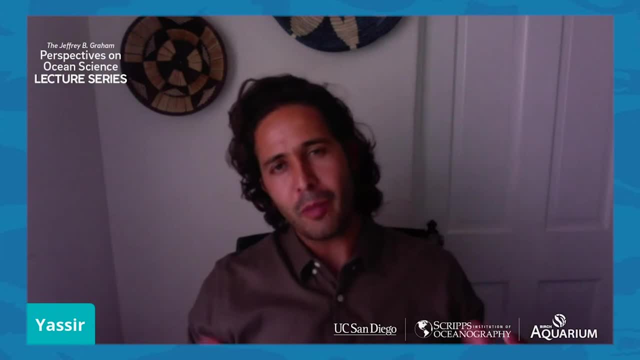 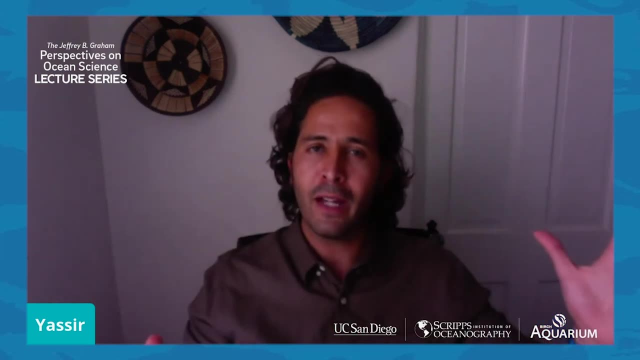 And that's one way that we can sort of think about the future, but that's a different analogy. It's an analogy that we can use in terms of what happens when you have these major, big hypoxic events, but the drivers are different. 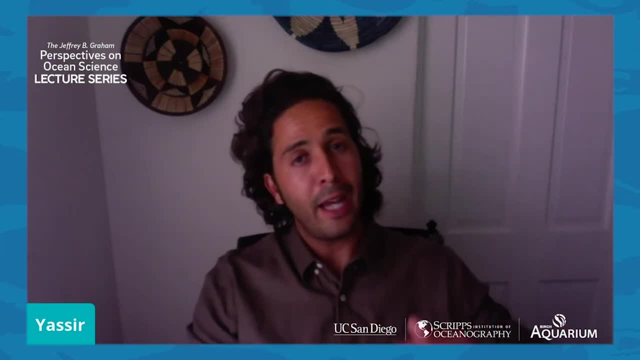 Those occurred over longer periods of time. They had much, much larger magnitude of warming and oxygen change, but they can still give us an idea about just sort of the impact on marine ecosystems and species diversity And they're very useful in that regard. So we can use them both as an analogy in terms of what happens when oxygen drops to very low level, but they're also quite different in terms of the mechanisms that were governing in the magnitude of oxygen change that were happening on those timescales.